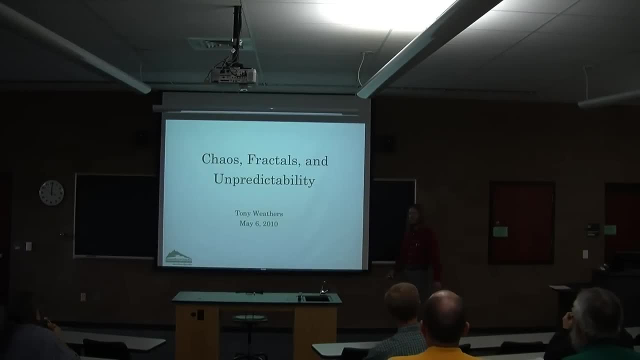 Thank you. Thank you for coming to hear what I have to say on this last talk of the year. So chaos, fractals and unpredictability- you've probably all heard about all three of those terms And I hope to give some clarification as to what a mathematician means when he or she talks about these things. 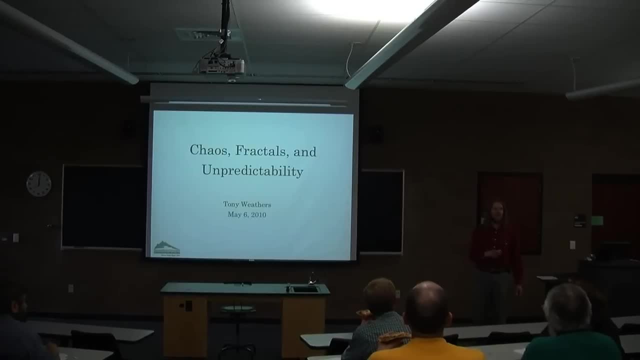 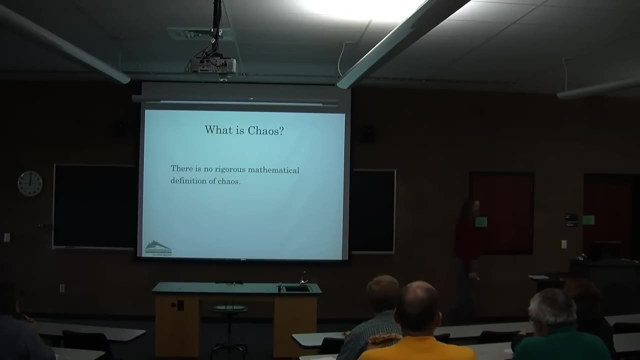 So perhaps we should start with a definition of what chaos is. but there isn't one, And that's somewhat embarrassing. It's not embarrassing to a mathematician. I mean, we pride ourselves on saying things precisely and rigorously. I mean, it's not like we're biologists or something. 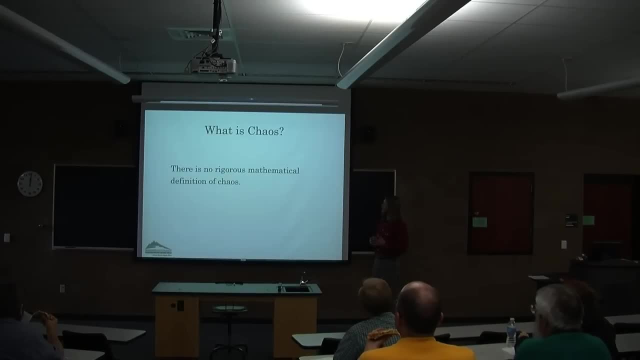 It's one of these things. I like to draw the analogy between chaos in mathematics and life in biology. I mean, if you go to a room full of biologists together and ask them to come up with a rigorous, precise definition of what is life, they probably couldn't. 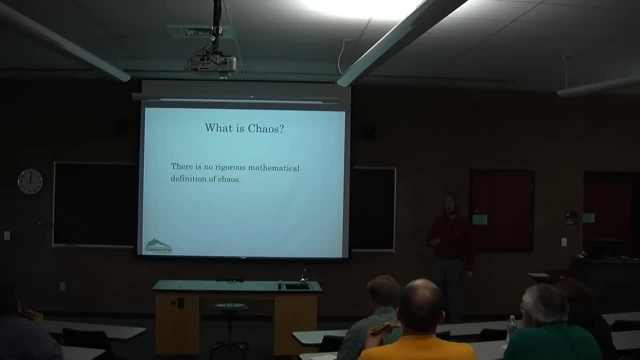 Now there are certain things that are considered hallmarks of life, And I hope to show you what some of the hallmarks of chaos are. But yeah, no rigorous definition. It's sort of like the Supreme Court case in 1964, Jacobelli versus Ohio regarding pornography and obscenity. 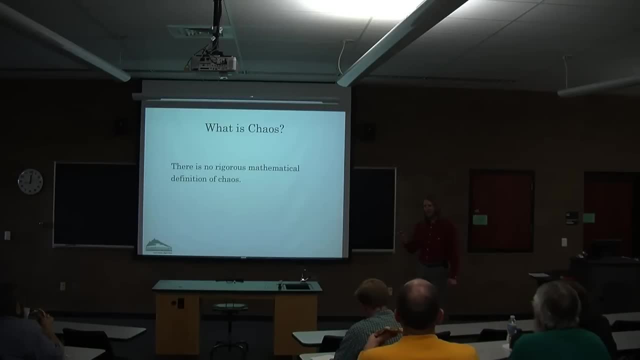 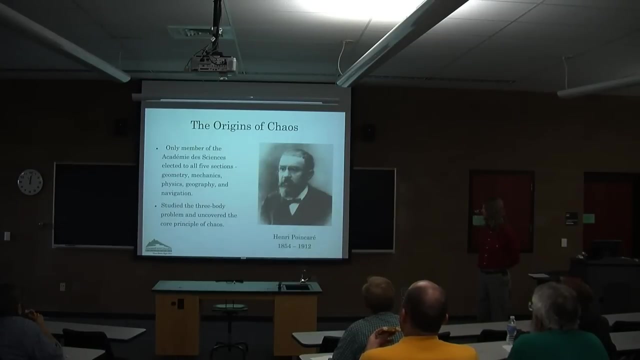 And the opinion written by Justice Potter Stewart was: well, we can't define it, but I know it when I see it, So presumably through years of practice. So let's see The origins of chaos. Chaos actually started way back in the 1800s with this guy, Henri Poincaré. 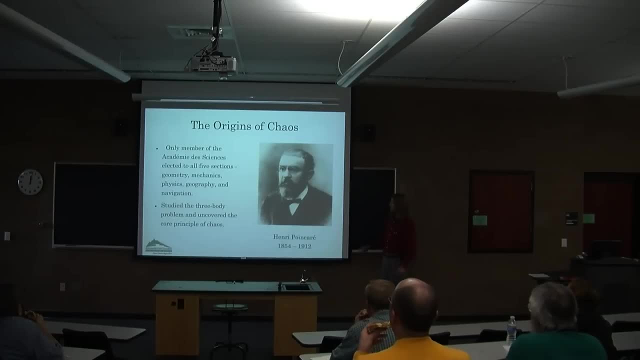 That's fun to say. He was quite a guy. He, as you see, was the only member of the French Academy of Science who was elected to all five branches, all five sections, And it was while studying the three-body problem in the 1880s that he discovered the principle that would go on to be recognized as the core principle of chaos. 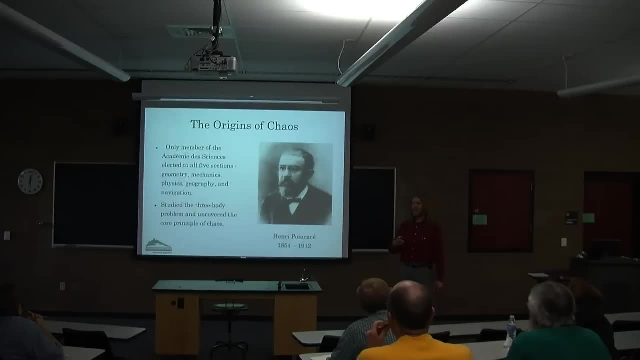 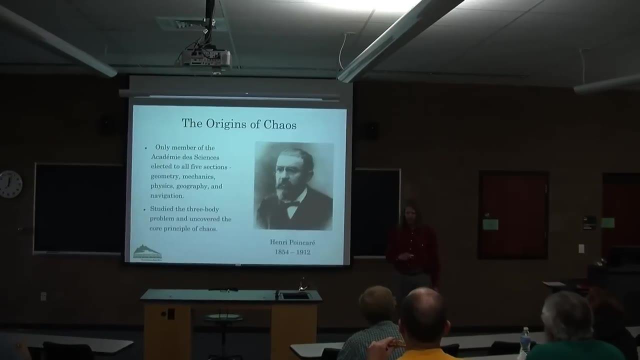 I bring this up not just because I like to say Henri Poincaré, But he also has one of my favorite mathematical quotations of all time, which is that mathematics is the art of giving the same name to different things, And it's very appropriate. 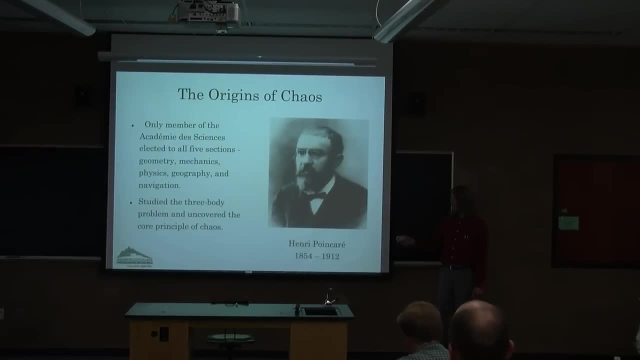 It's very appropriate in this situation, because it wasn't until almost 100 years later that people started studying chaos and realized: oh, wait a minute, This is the same thing he was doing back then. Right, Different things, same name. So who did discover chaos? 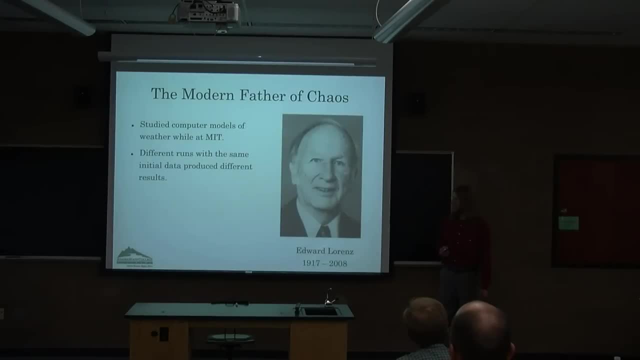 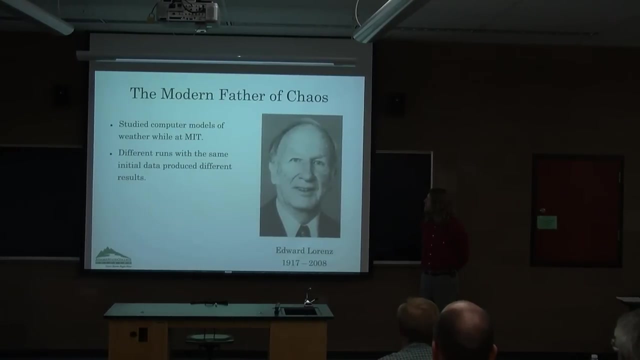 Well, the guy who gets the most credit for chaos is this guy, Edward Lorenz, And he was a mathematician working at MIT in the 50s and 60s And he was doing computer simulations of weather And he found that when he did different runs of his model with the same initial data, he got different results. 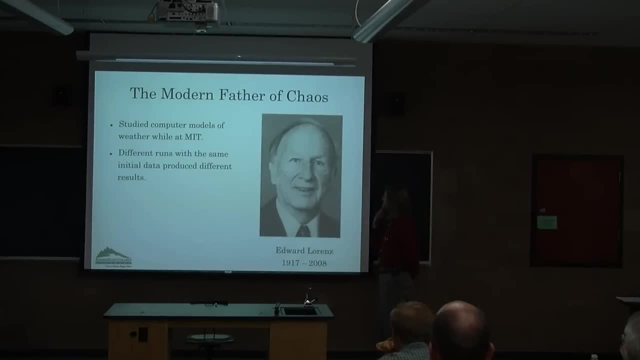 Well, I should say it wasn't quite the same initial data. But what he had done was he had run these computer simulations and saw some interesting long-term behavior that he wanted to study further. But he didn't want to start his simulations over at the beginning to let them run all this way. 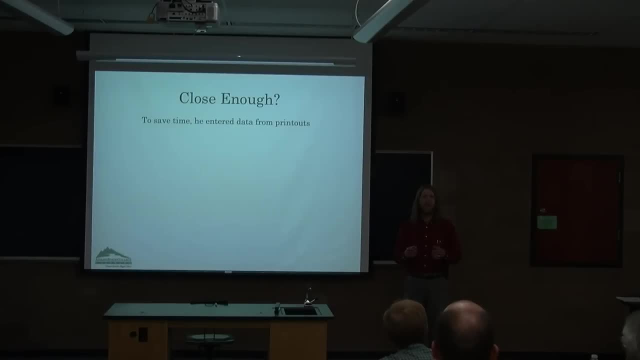 So he would just grab printouts of the data from somewhere in the middle and put that in and see what happened. He didn't really. I mean, he had to save time here. MIT had state-of-the-art computers in 1961.. 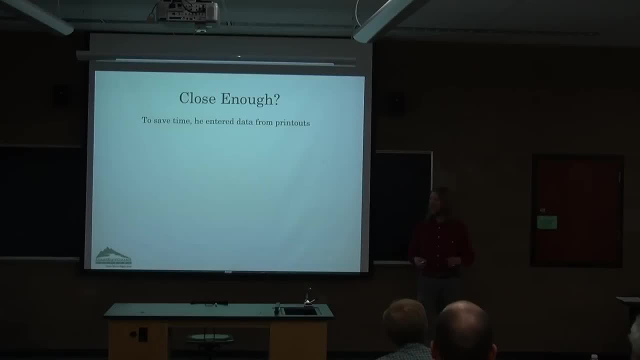 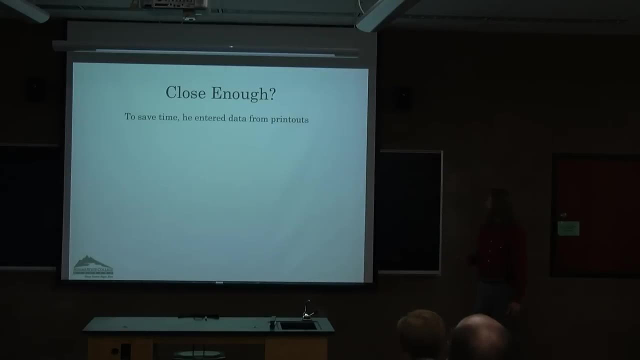 But it was 1961. So computing power, state-of-the-art, was slightly faster than a trained monkey with an abacus. So he went, grabbed his printouts and typed in some data And on the printouts he saw the number 0.506.. 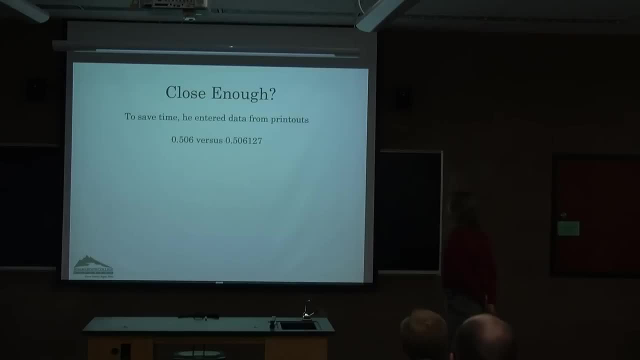 And he typed that in and let it go. The problem was that wasn't really the number that the computer had in mind. The computer knew 0.506127. And to save space on the printouts, they only printed three decades, So he wasn't really putting in the same data. 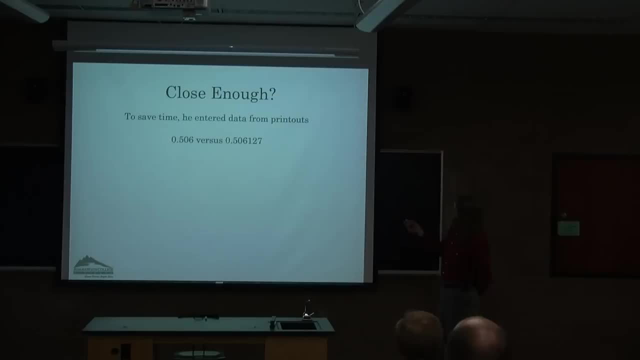 But I mean, how much difference is there? here We're talking, what is that? ten hundred thousandths, Millions? Not much at all. It shouldn't make a difference, But it did. Here's one of his graphs from some of his data: 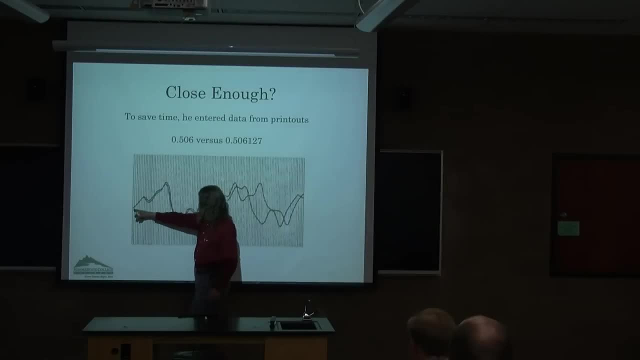 And what he saw was: initially it looked pretty good, They tracked each other pretty well, But then, as time went on, things started diverging wildly And in the long-term it didn't. In the long-term they didn't look anything alike. 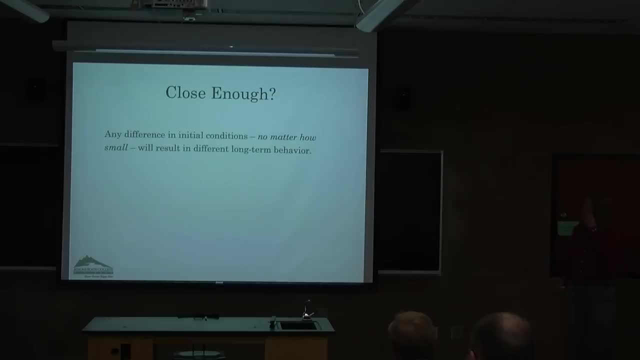 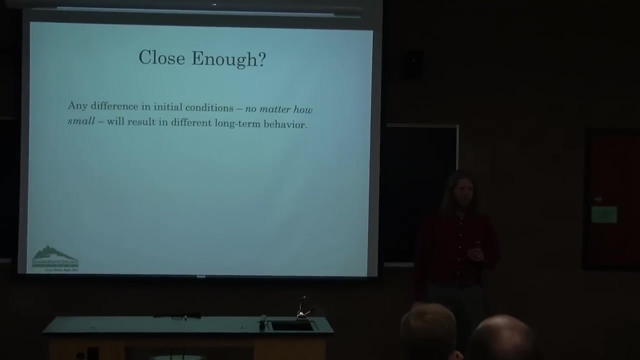 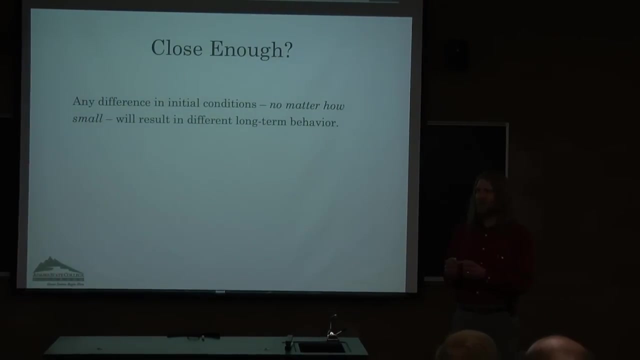 So what he discovered was that any difference in the initial conditions didn't matter how small any difference whatsoever would result in different long-term behavior, Often very different long-term behavior. This was quite contrary to the thinking at the time Most people, even in your daily life you're used to making a little bit of tweak in the initial conditions. 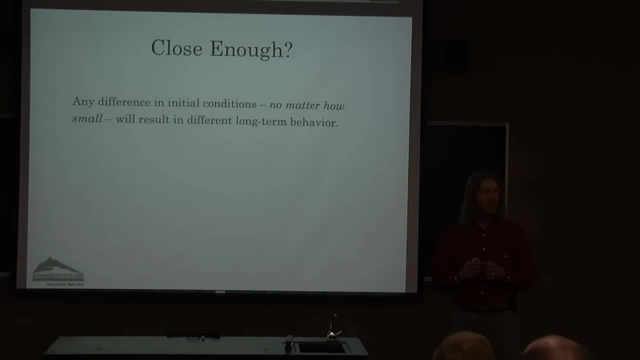 And it doesn't make that much difference in the outcome. If you put an eighth of a teaspoon of salt into your recipe instead of a quarter teaspoon of salt. it's not going to make it blow up on the stove or something. It's not going to be that drastic a difference. 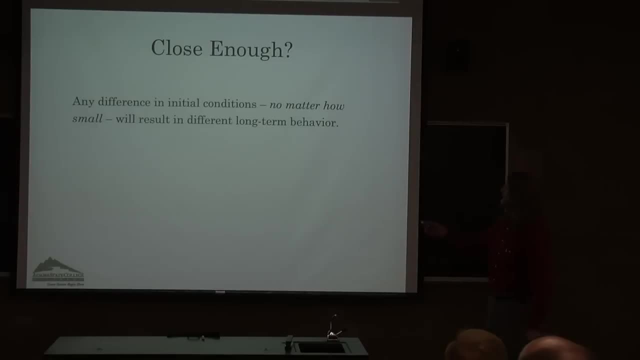 But it was, And so this encapsulated the core principle of chaos, which mathematicians like to call sensitivity to initial conditions. It doesn't matter how small a difference you start with in some systems, in most systems, it will make a big difference in the long run. 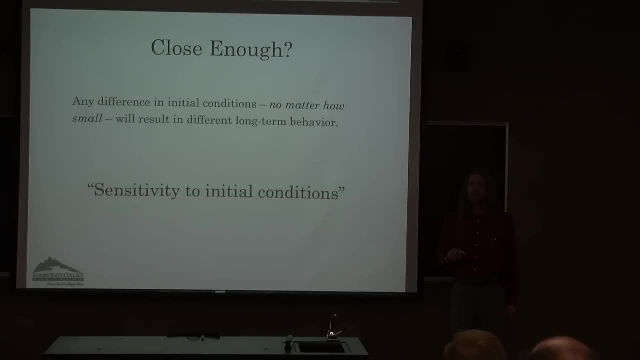 Now, he was studying weather, And so it's reasonable to ask: what does this mean for weather? Well, for one thing, it meant that long-term weather forecasting is doomed. There's no way you can successfully do long-term weather forecasting. 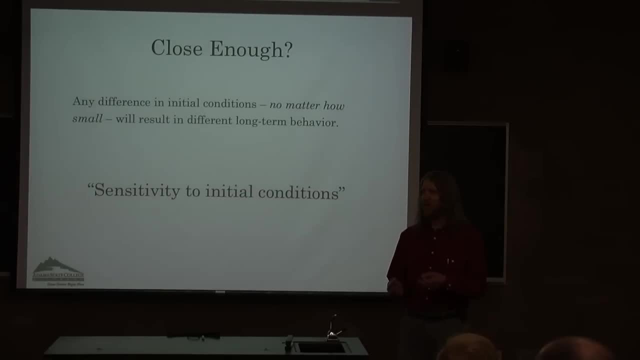 Now let's think about why that is. What do weather forecasters have at their disposal? Well, they get data. Where do they get data They get from? well, for instance, out at the airport. they have thermometer, wind speed anemometer. there we go. fancy word: hygrometer. 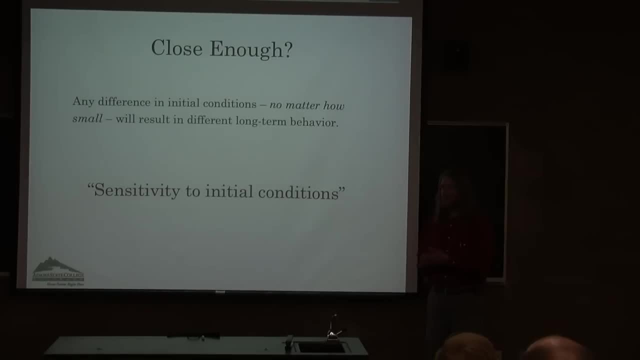 So they know all these things about wind speed, temperature, humidity, but they probably don't know the exact temperature. But let's just fantasize that they could. They have a thermometer that will read the exact temperature. They can tell the exact humidity. 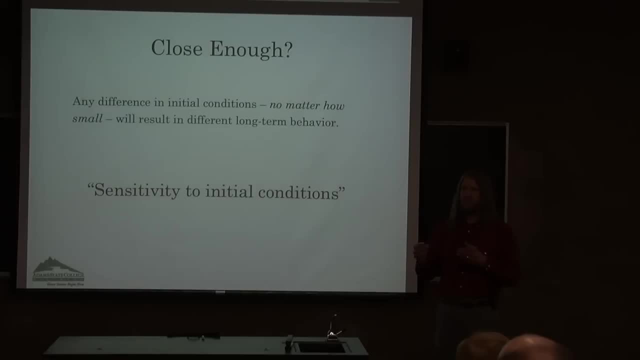 They can tell the exact wind speed. Well, but how far apart are these sensors? I mean, just because you know the exact conditions out at Alamosa Airport doesn't mean you know the exact conditions out in front of Richardson And for the same exact set of conditions at the airport. 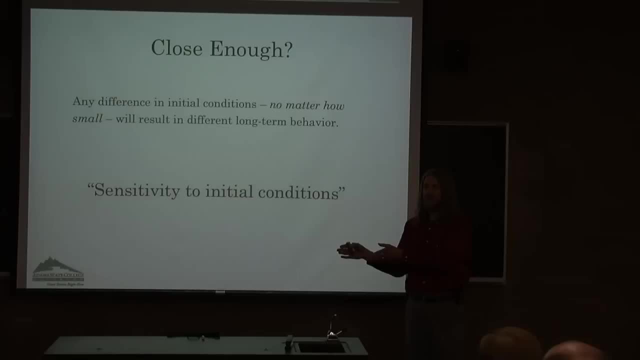 you could have vastly different conditions over in front of Richardson. So what could you do? You put more sensors. Well, how many is enough? Suppose you put a grid- A grid whose spacing is one foot- all over the surface of the Earth. 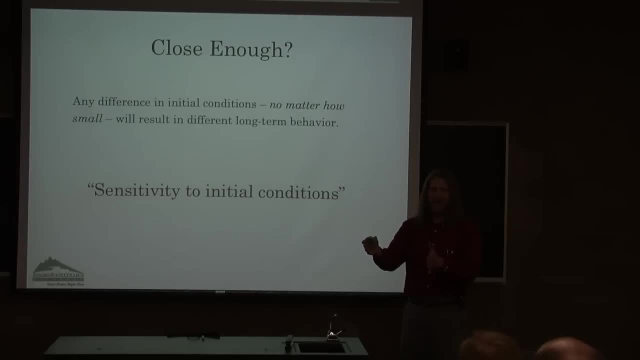 You put a sensor every grid point. Well, that's still not enough, because, well, now, you don't know what's happening between the sensors, You don't know what's happening up here, So you'd literally have to fill all of space with sensors, perfect sensors. 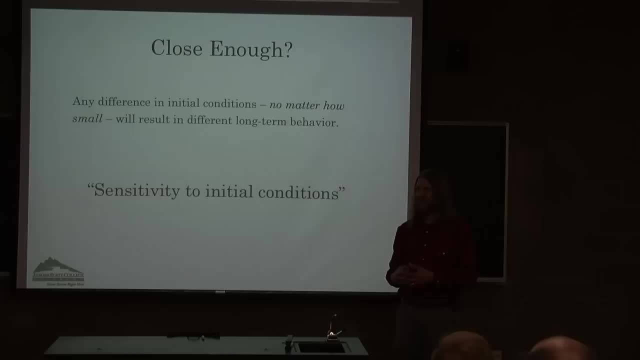 Well, but even then, that's still not good enough, because how big are they? Well, they're a micron. Well, but you don't know what's going on in between there, okay, So long-term weather forecasting is impossible. 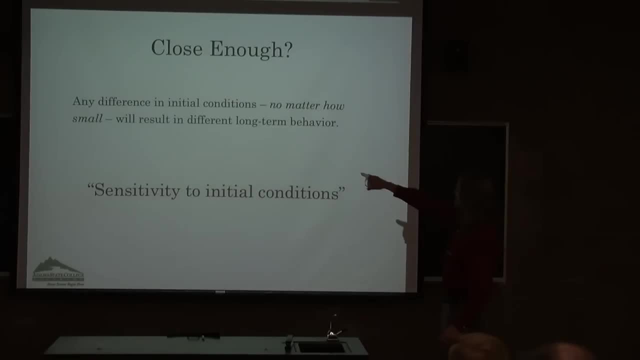 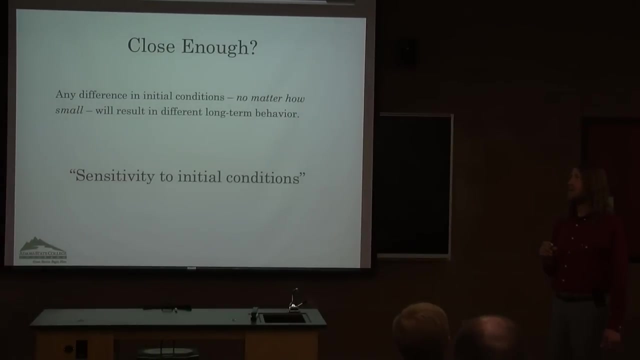 But even worse, small disturbances, small differences in initial conditions can make very big differences in outcomes. In 1972, he gave a talk. he, being Lorenz, gave a talk at the American Association for the Advancement of Science, And the title of his talk has come to be: 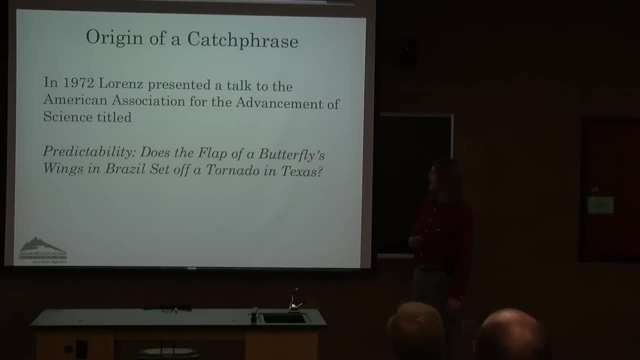 contain the catchphrase for all of chaos theory. I'll let you read that. Because if no difference in initial conditions is too small, well, a butterfly flapping its wings makes a little disturbance in the air. Maybe that disturbance in the air six, eight weeks later. 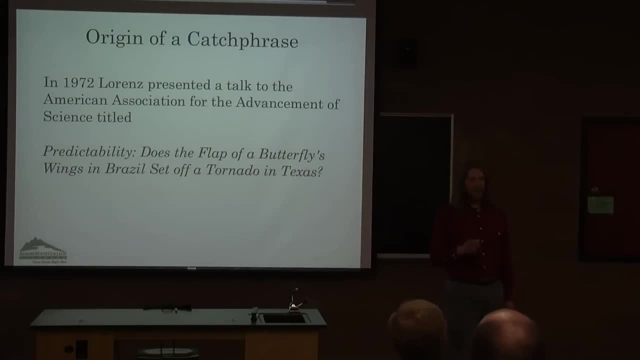 can make a tornado somewhere else in the world, And so the thing you'll hear, the catchphrase that you hear in reference to chaos, is the butterfly effect. You hear that a lot. butterfly effect. Butterfly flapping its wings in Japan and make a hurricane in the Atlantic. 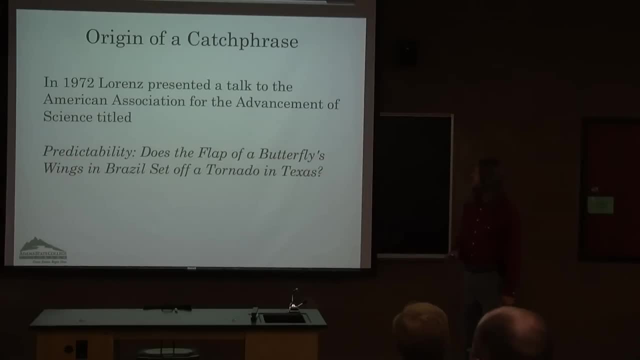 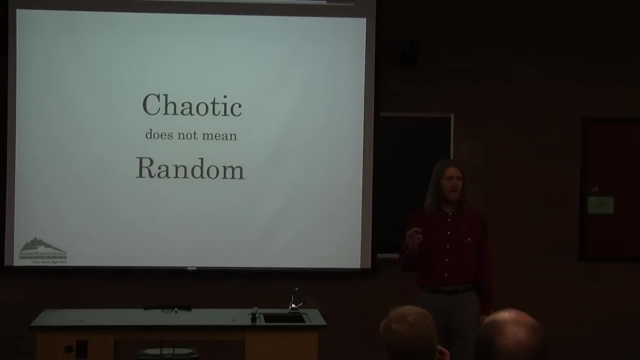 six weeks later, Who knows? Now here's one thing that I want to make sure everybody gets out of this talk: Chaotic does not mean random, okay. Long-term weather forecasting is not possible. Long-term weather is unpredictable. That doesn't mean it's random, okay. 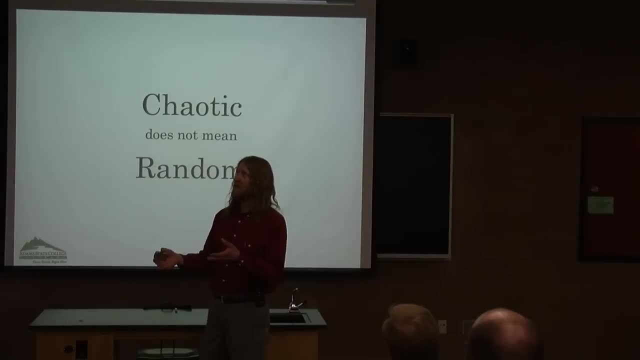 I can't say whether on July 15th it's going to rain or not, or be windy or not, or whether it's going to be 73 degrees or 84 degrees, But, barring some sort of global catastrophe, I can say for certain that the high temperature will be above zero. 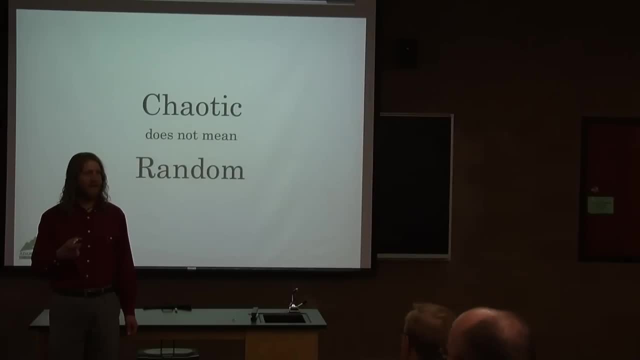 Okay, In fact, I can tell you that a week from now, the high temperature is going to be above zero. Okay, So it's not random. It's not like you're going to have sleep one minute and then thunderstorms the next. 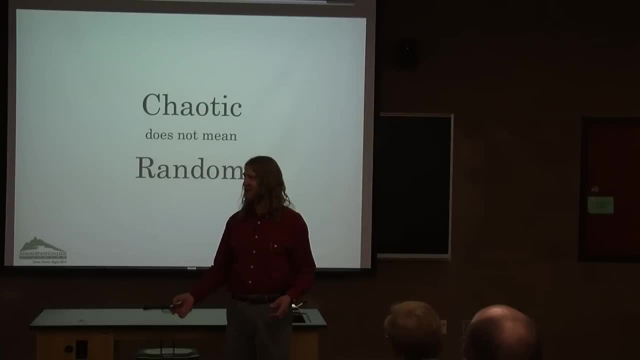 and then 117 degrees and sunny the next minute. right, It's not random, It's chaotic. And there's a difference. Chaotic means unpredictable within a certain range of parameters, Okay, Not absolutely random. So what does chaos have to do with fractals? 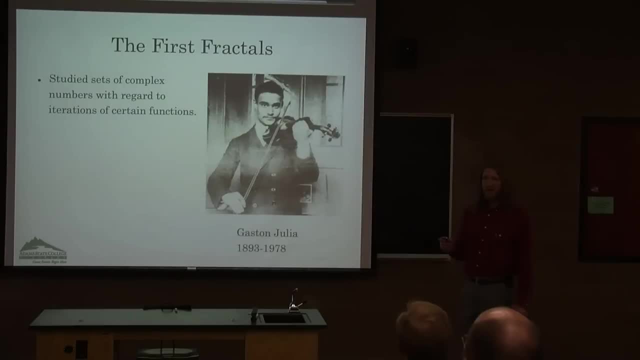 I'm glad you asked. So the first person who investigated something that we would recognize today as being fractals was this guy, Gaston Julia, And what he did is he looked at complex numbers and he looked at sets of complex numbers. 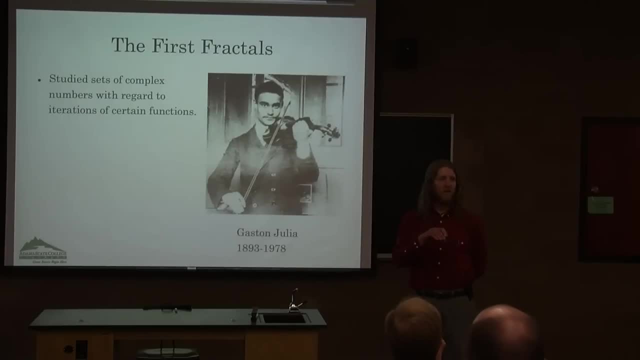 and what happened to numbers in these sets if you took some function and iterated it on these numbers over and over again. Okay, So let's look at a very simple example. Oh, I was going to say a couple of words. When you look at these guys in math history, 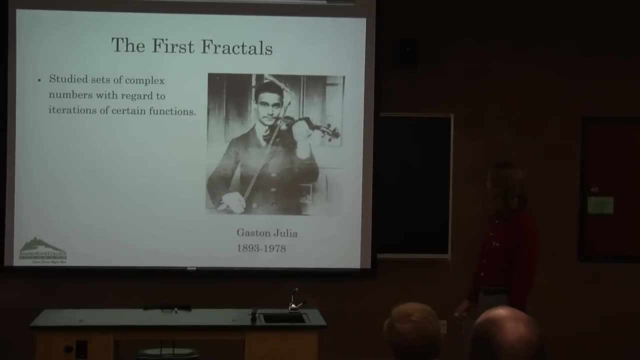 it can be quite intimidating, quite a shock to the ego. I mean, Julia, here was quite a guy. He was a good, quite a good violinist. He, let's see, when he started fifth grade they had moved to a new country. 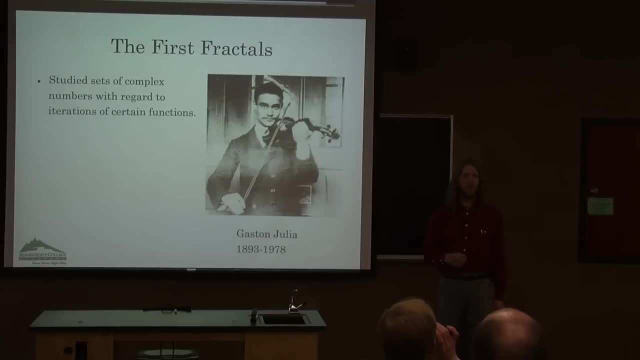 They moved and the school was in German. He'd never studied German, so he basically learned German in a month on his own, went to school. By the end of the year he was the top student in all subjects, including German, in the school. 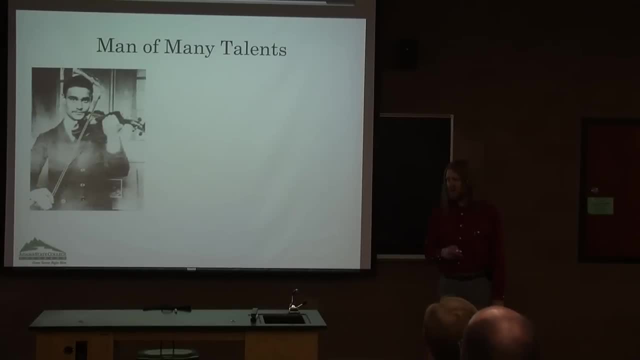 Interesting guy. He was working in France during World War I. At the outbreak of the war he was drafted And so we can see hello, There he is in his garb, And even in the Army he excelled, showed leadership and bravery. 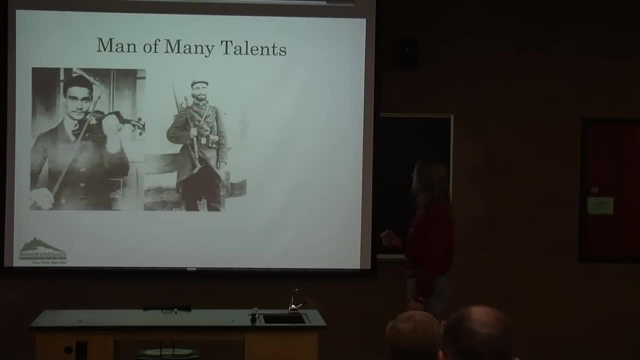 well, above and beyond the call of duty. But unfortunately he also displayed an uncanny ability to stop bullets with his face. And yeah, ow, If you look at that, I don't know that's pretty gruesome, but it didn't stop his productivity. 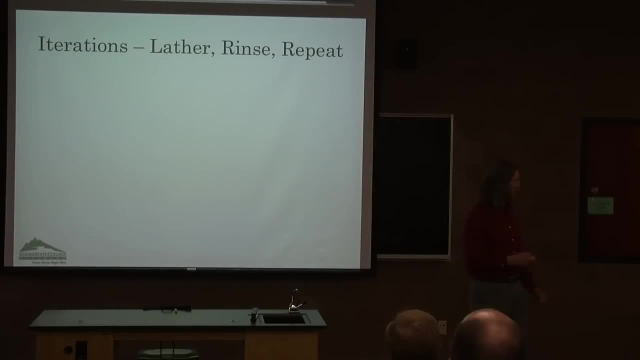 So anyway, let's go on to iterations. What are iterations? Like it says on the bottle of shampoo: right, Lather, rinse, repeat. If you need instructions on your shampoo, you have bigger problems than dirty hair. Of course, the other problem. 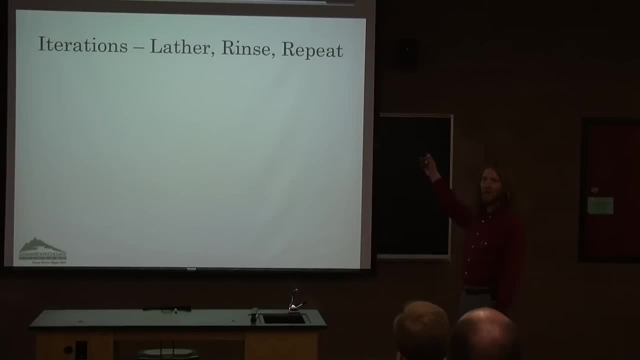 and the computer folks in the audience would appreciate this. you get stuck in an infinite loop in your shower. Just lather, rinse, repeat, lather, rinse, repeat. You never get out of the shower. Well, I guess that sort of implies. 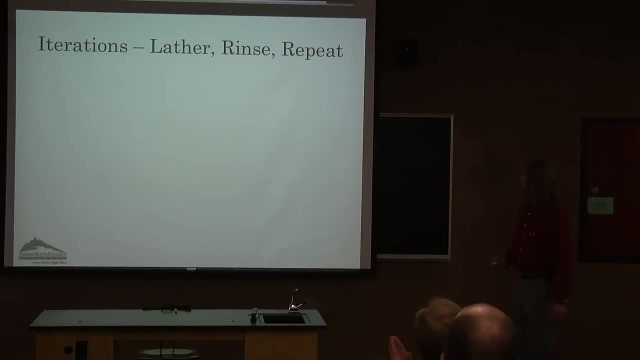 that computer programmers take showers, But anyway. so let's imagine an iterative sequence. We're going to take a number, x, Say, for instance. we'll start with two x sub zero. x not equals two, And from then on 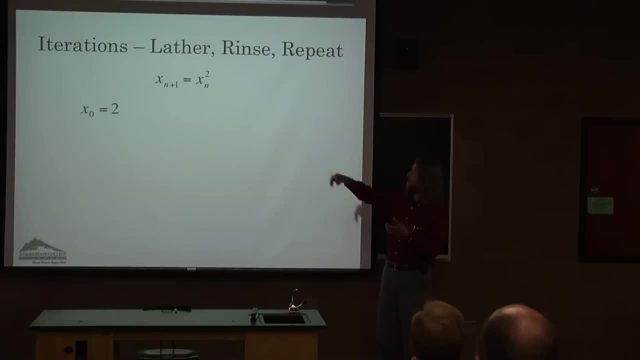 we're going to find the next number in the sequence, in this case simply by squaring its predecessor. So you start with two, square that you get four, 16,, 256,, et cetera. So that would be an iteration. 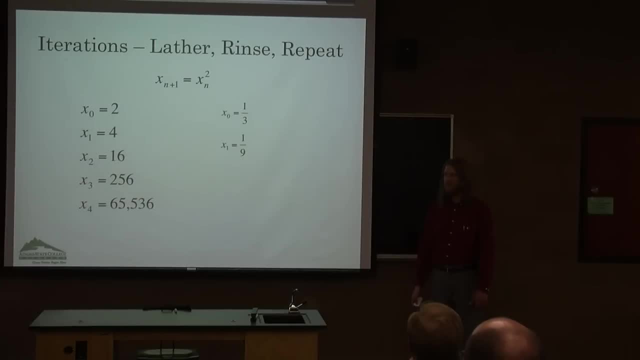 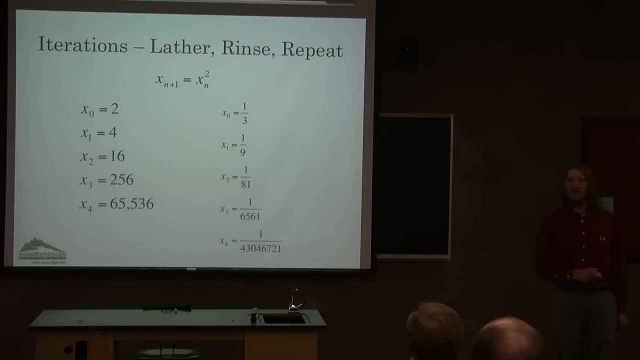 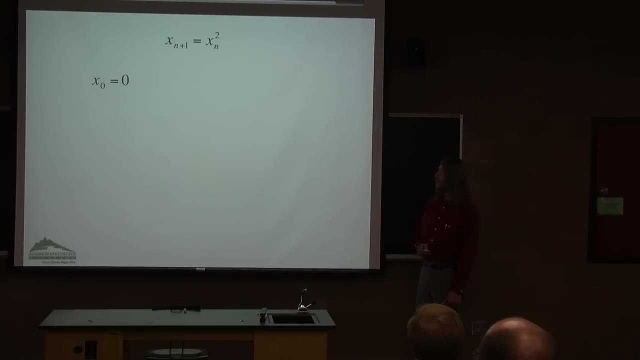 There are a couple of special numbers with respect to this particular iteration, one of which is zero, Because you can convince yourself pretty quickly that if you square zero, you get zero, And then you square that, you get zero, and zero and zero. 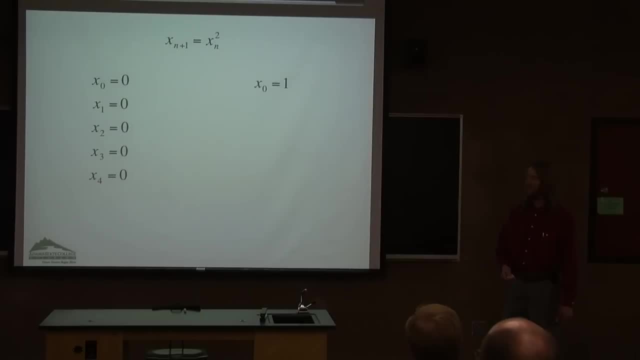 Same thing happens with one. Take one square it, You get zero. or one, One, one, one All the way down the line. Now you'll notice I didn't really say anything about negative numbers. There's really no reason to talk about negative numbers. 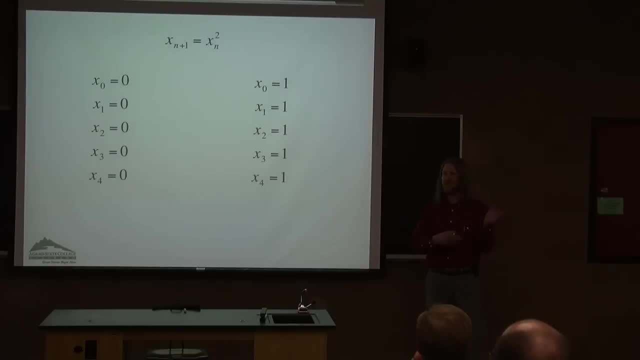 in terms of this thing, because as soon as you square it the first time, you're dealing with positive numbers. But let's look at what happened. What we saw is that when x not was zero, well of course it stayed at zero the entire time. 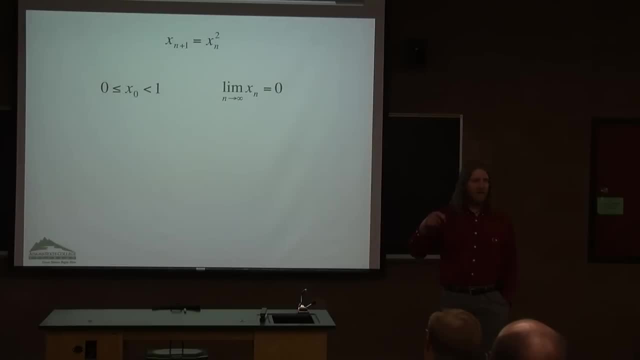 If it was between zero and one- the example was a third- then the more you square it, the smaller and smaller it gets, And so any number between zero and one, including zero, has the property that in this iteration the limit is zero. 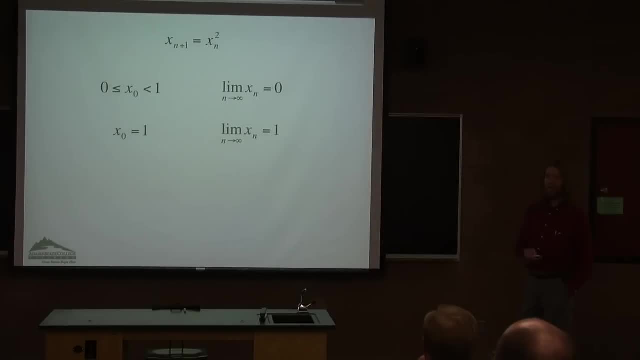 And then there's that special guy one, and he just stays at one forever. And if you take a number larger than one, then you find that as you iterate the thing over and over again, it gets bigger and bigger and bigger without bound. 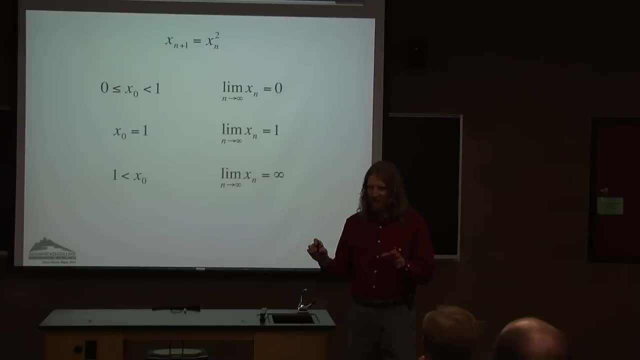 So what I could do is I could draw a picture on the number line and I could draw in one color all the numbers that don't blow up to infinity under this iteration, and then a different color for the ones that do, And what you would see is a picture. 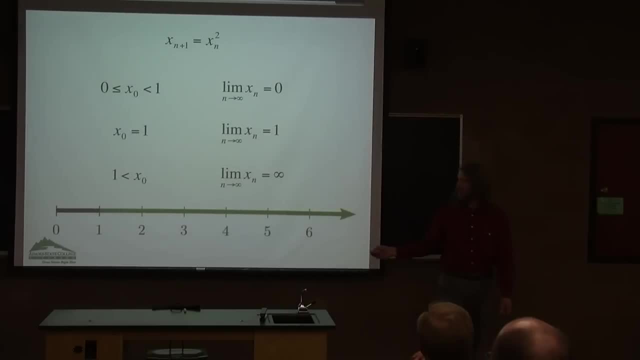 something like this: All the numbers in here between zero and one either stay put- that's what zero and one do- or they go down to zero, But they stay bounded. They don't blow up Anything larger than one. if I iterate this over and over and over again, 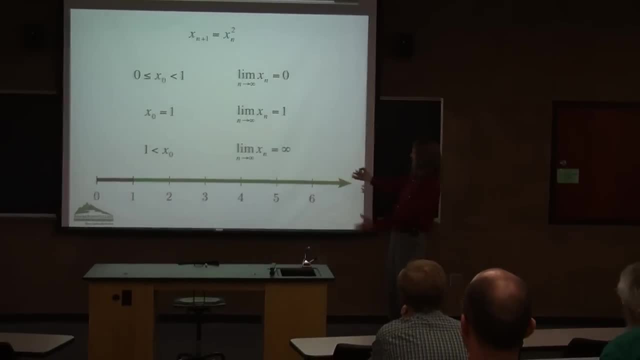 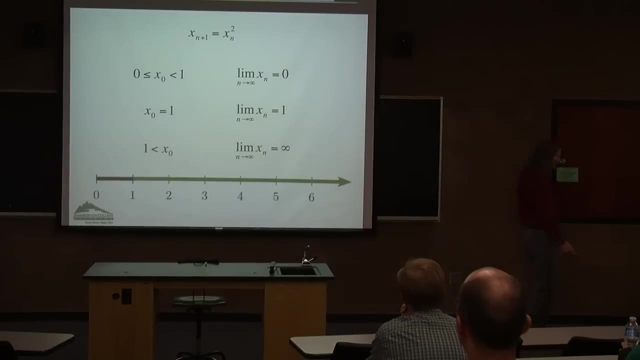 it blows up, It goes off to infinity, And so this, well, there's sort of a picture like these fractals that we're going to look at. So what Julia did was, well, he worked with complex numbers, Because remember what I said here: 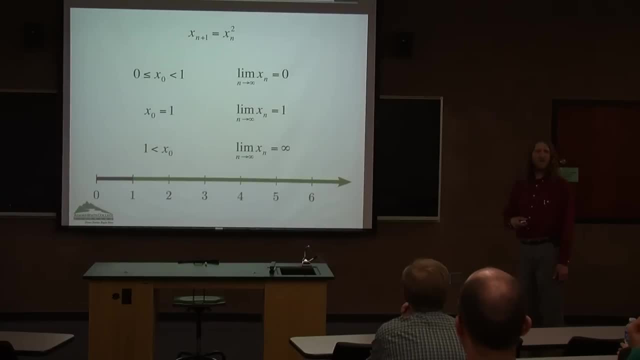 about. if you square a negative number now, you're off into the positives and you're there forever. Well, real numbers aren't that interesting in these sort of iterations. So he looked at complex numbers. So what are complex numbers? Complex numbers look like this: 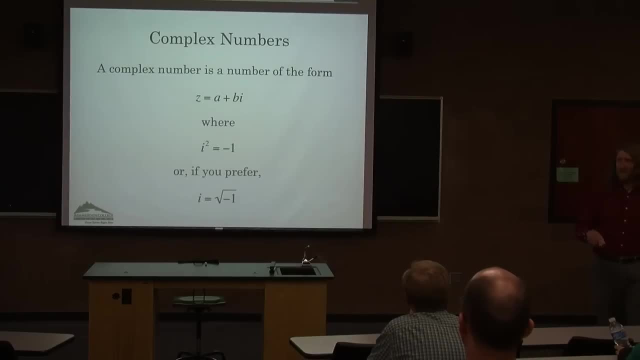 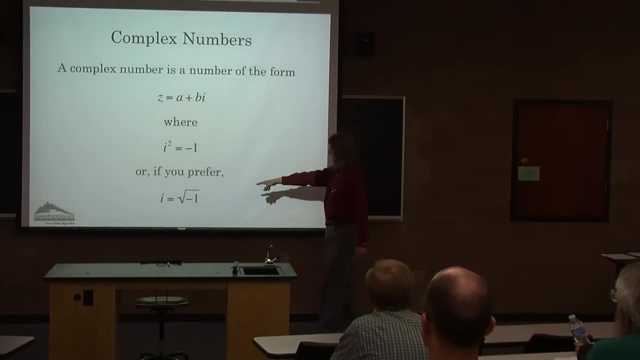 a plus bi. a and b are real numbers and i is this special imaginary unit. It has the property that it squares to be minus one or, if you like, you can think of it as the square root of minus one. It's an unfortunate consequence of the nomenclature. 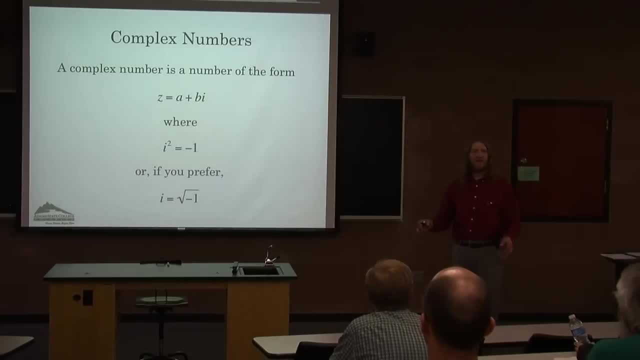 that people think: oh, imaginary, it's just this thing out there. There's really no such thing as imaginary numbers. Well, okay, then what is two? All numbers can be thought of as imaginary. What's a three? What's minus seven? 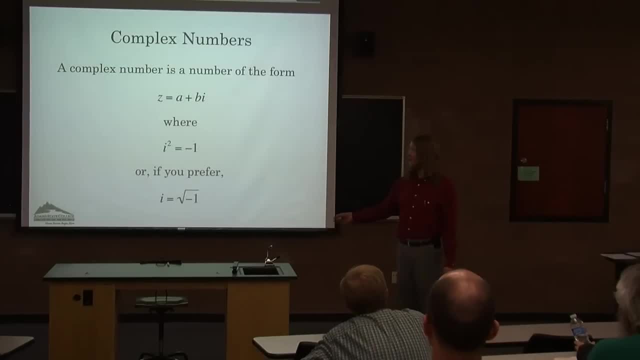 So it's as valid a number as any other number is, And it has some really interesting properties, not the least of which is this fact that when you square i, you get minus one- So complex numbers. we generally try to think about those as points in the complex plane. 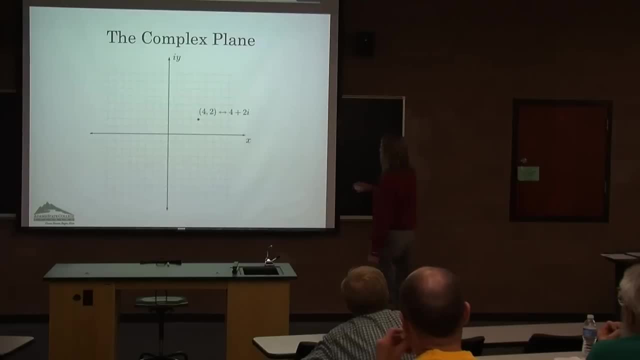 So we identify a complex number a plus bi with the point in the plane a comma b, So for instance the complex number four plus two. i I would think of that as the point four comma two in the complex plane, The difference between the complex plane and the real plane. 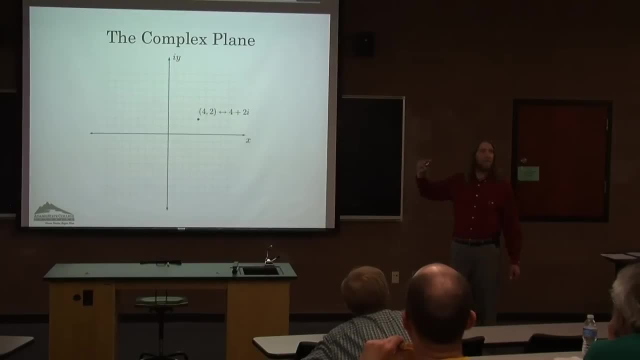 of course, being the fact that this isn't just y, it's i times y. All right, Well, complex numbers do really interesting things when you multiply them. For instance, suppose we took four plus two i and multiplied it times this one minus i. 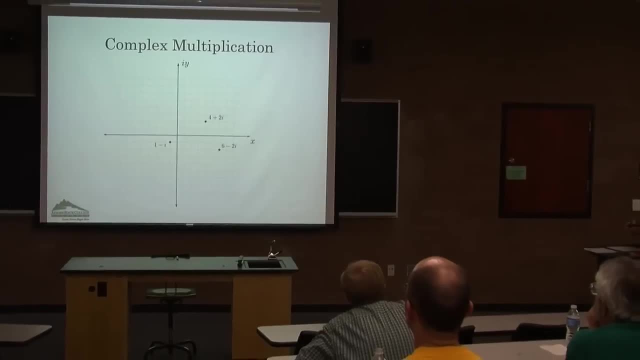 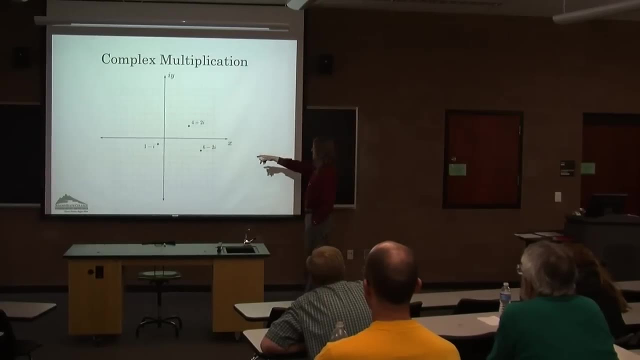 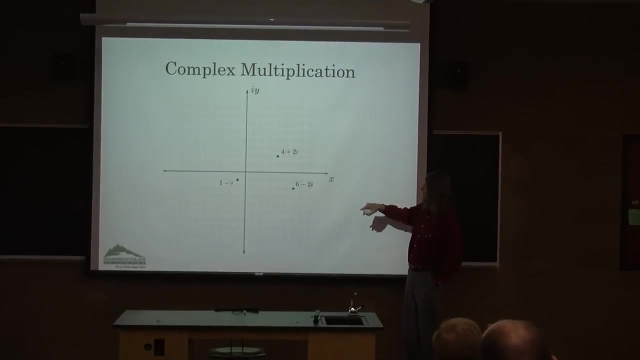 What you get is six minus two i, And it's not exactly clear why, in terms of the picture, why you would get that. You can express it in a nice geometric way: It has to do with the angles that go through them and then adding the angles to get this. 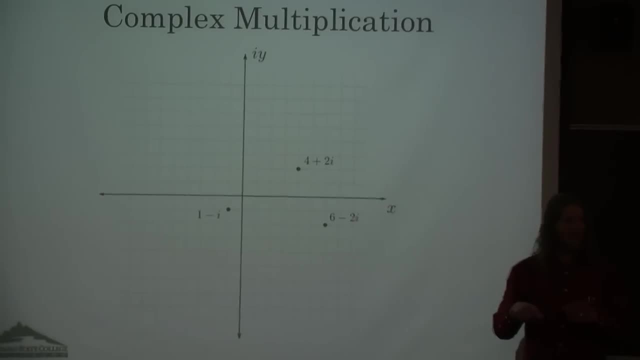 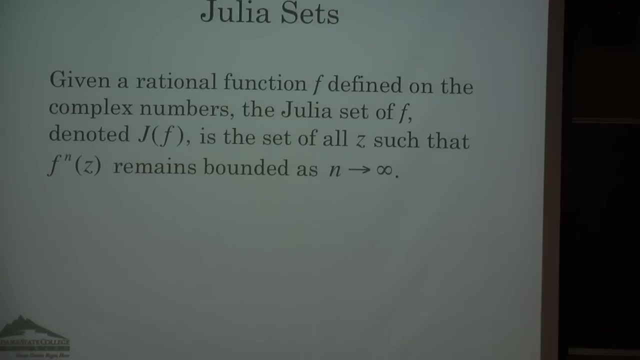 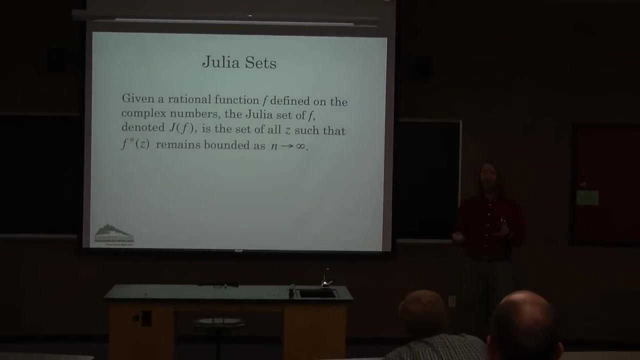 But the point is that complex multiplication results in much more interesting behavior than just real multiplication. All right, So what Julia did was this. He said: take a rational function. for those of you who care, A rational function is simply a quotient of a polynomial. 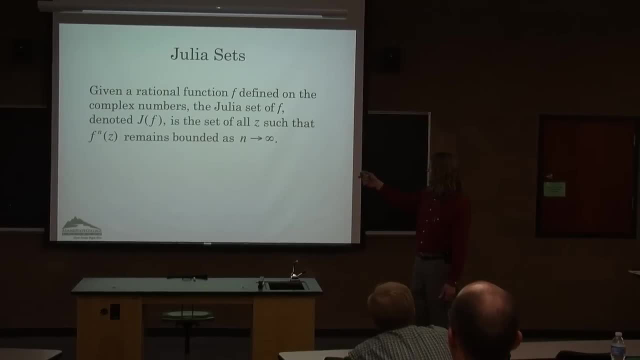 A polynomial or a polynomial, And he looked at this set that he called j of f, the Julia set. I doubt he called it that, but subsequent people have. Okay, The Julia set of that function. f was the set of all complex numbers. 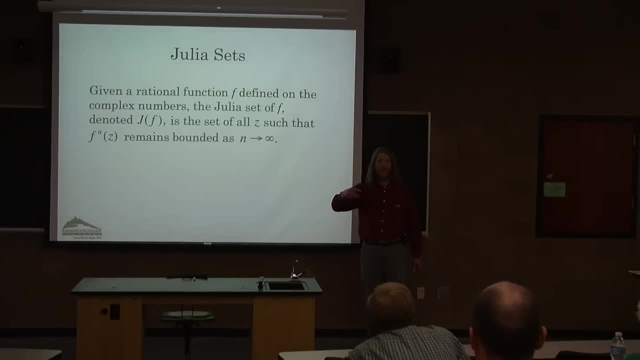 such that if you iterate this function over and over again, those numbers, well, they don't necessarily stay put, but they don't blow up. Okay, They might be something that goes to zero, It might be something you'll see- a lot of cycles. 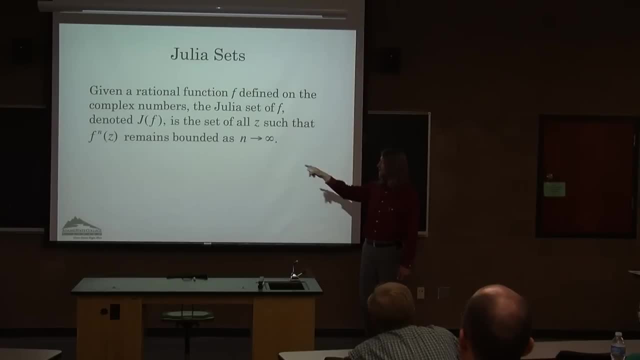 in some of these sets, Okay. But basically, if it blows up, if f n of z as n goes to infinity, you have some z, you iterate the function over and over. If that thing keeps going bigger and bigger and bigger, 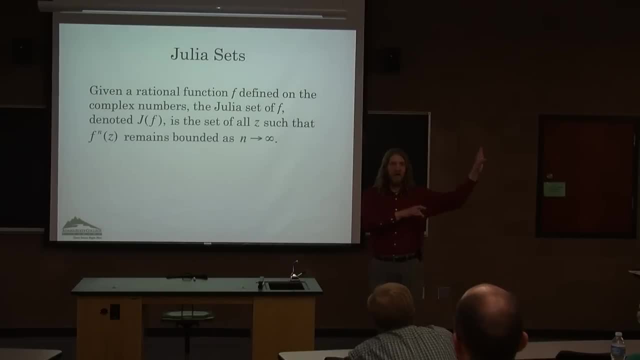 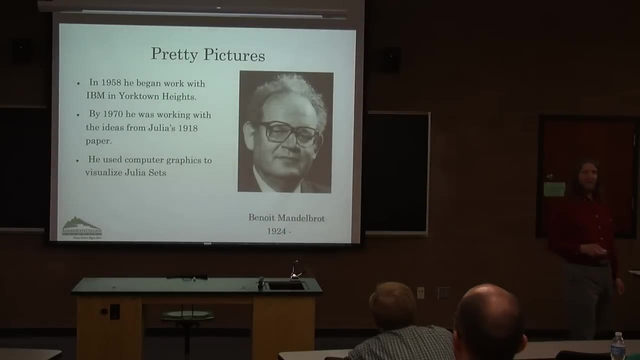 blowing up. that's not in the Julia set, Okay, Everything else is So. now, along came this guy, Benoit Mandelbrot, And he was working at IBM starting in the late 50s And by 1970,. 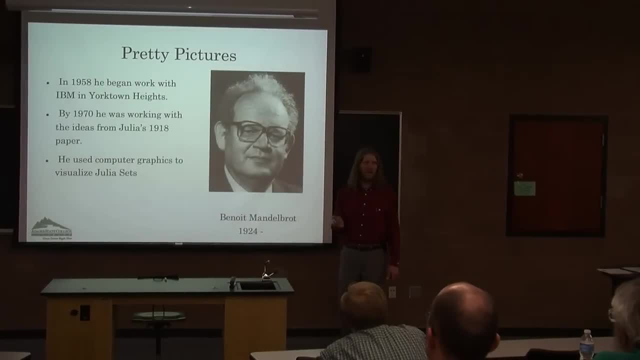 he got hold of some of these ideas from Julia's paper in 1918 where he did these Julia sets, And he had an advantage that Julia didn't, And the advantage, of course, was computer graphics. Okay, And by 1970,. 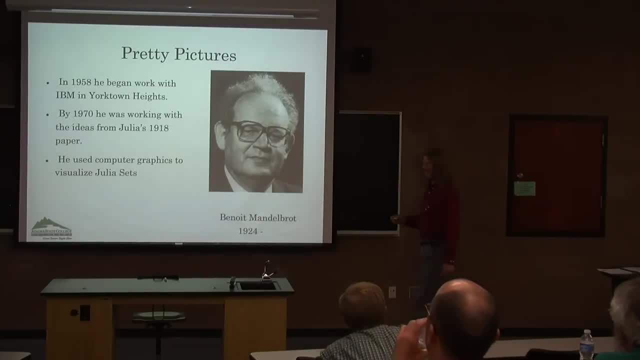 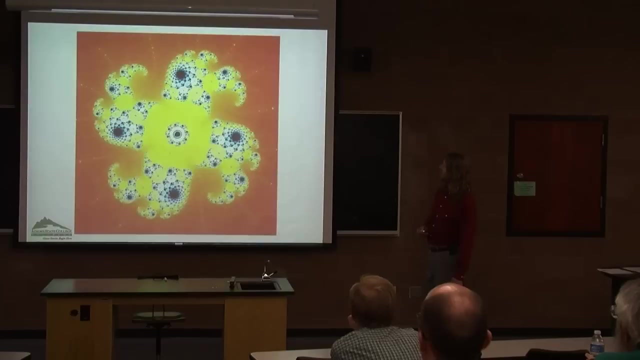 two trained monkeys with an abacus. Okay, So he used computer graphics to visualize these Julia sets and came up with all the kind of pretty pictures that you guys are probably somewhat familiar with. Okay, Well, like this: Ooh, And this: 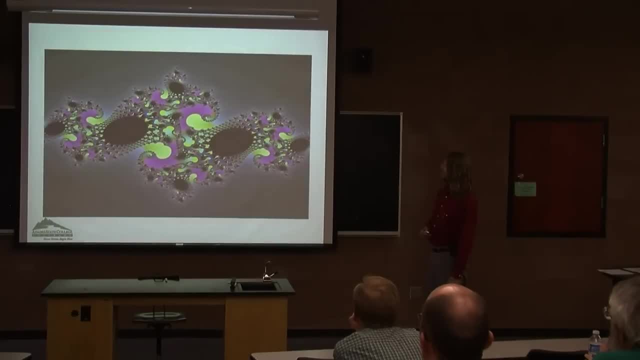 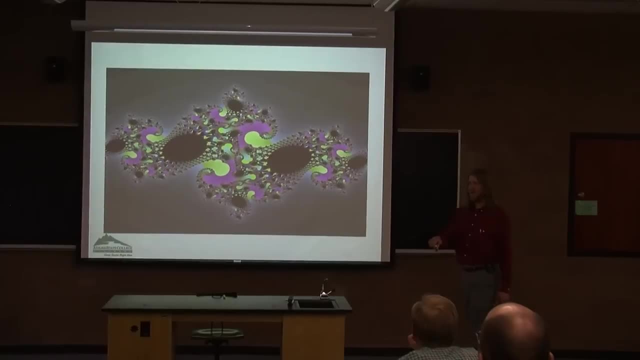 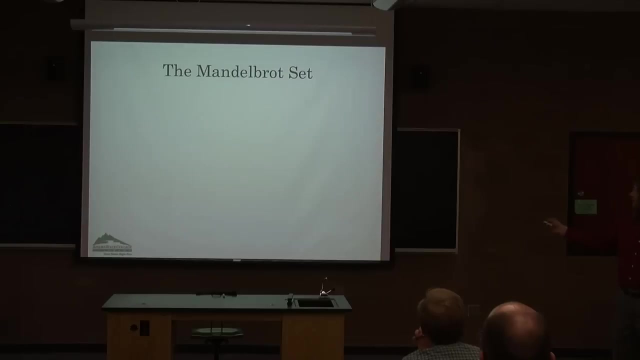 This And this. So, but he is most known, of course, for one specific set that he worked with, which has been dubbed the Mandelbrot set. The Mandelbrot set took a very specific function. this one right here. 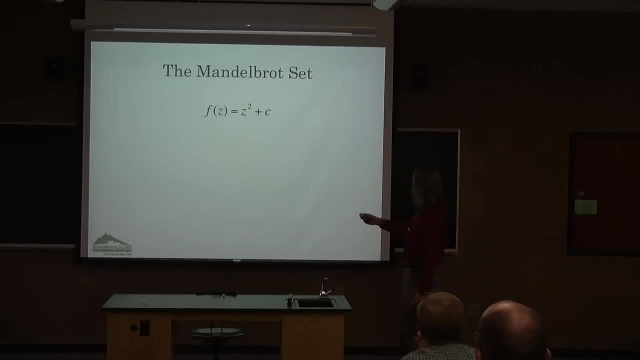 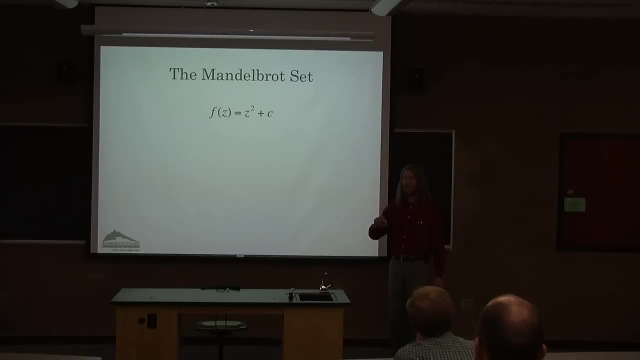 Take a complex number, Z, Okay. And then you take some other complex number, some constant, called C. Often you hear this referred to as the seed. The seed is the seed of this function. And you take the number Z, you square it. 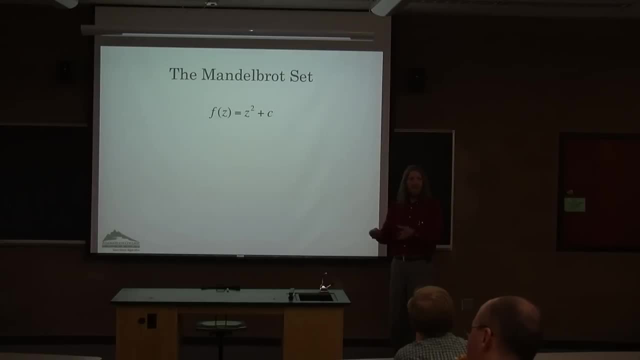 and you add C Square, it add C Square, it add C, And that leads you to an iterative sequence like this: Okay, So pick some Z, call it Z naught, and then you do this. Now, the thing about the Mandelbrot set is he picks it. 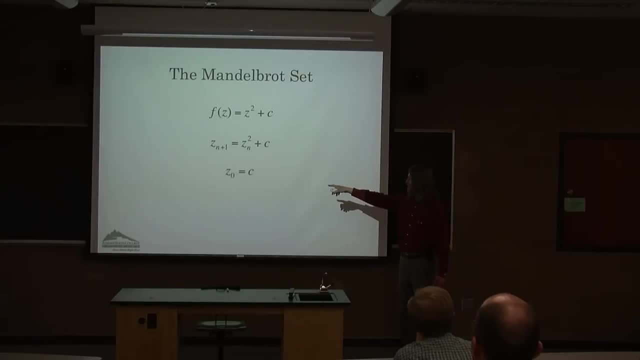 in a very specific fashion. Okay, His first element of his iterative sequence is the number C itself. Okay, So take C square. it, add it to itself. Square that, add the C Square. that add the C Square that. 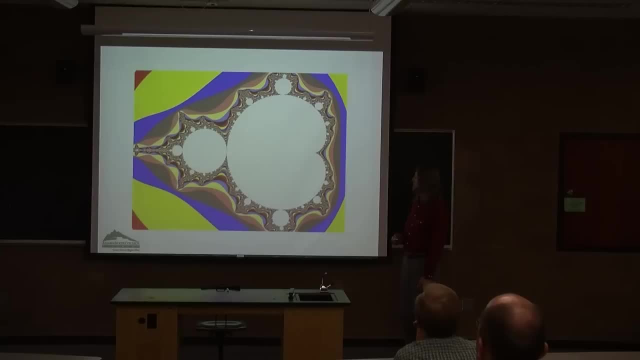 add the C. Okay, What happens? Well, what happens is you find that and the coordinate axes are not on here, but the coordinate axes go basically right through there and right up through there The white designates the points that are in the Mandelbrot set. 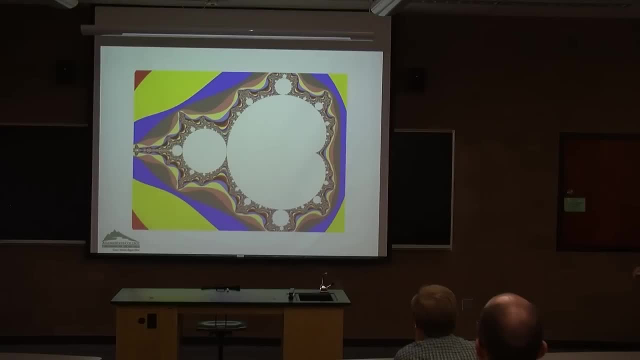 Okay. So those points you do this iteration over and over again, those points do not blow up to infinity, They stay bounded, Some of them go zero, some of them go into cycles: a, two cycle, three cycle, five cycle. 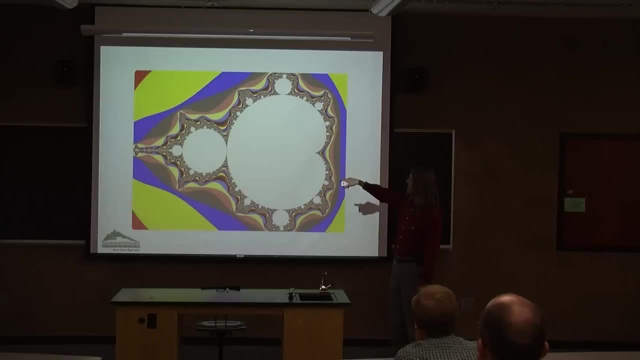 Okay, Some of them bounce back and forth in there in a non-cyclic fashion, but again, they don't blow up to infinity. The ones that are in color do blow up to infinity and they are colored by how rapidly they blow up to infinity. 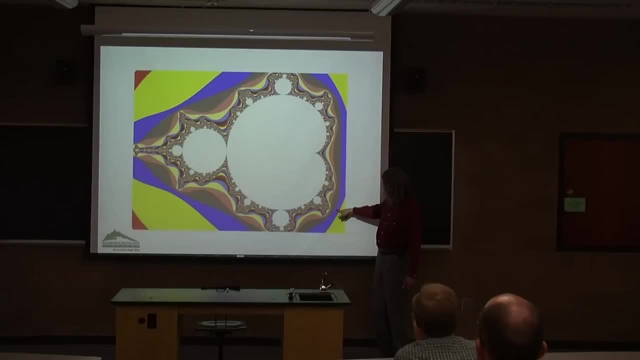 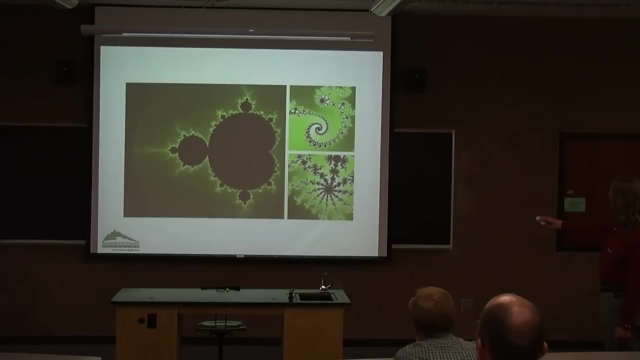 Okay. So these guys blow up much faster than these do, than these do, than these do, and then things get a little, a little hard to tell what's going on. Okay, Here's another representation that shows some, some zooms in on the various parts of the Mandelbrot set. 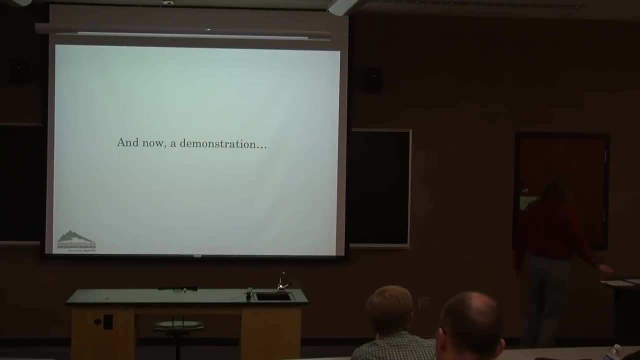 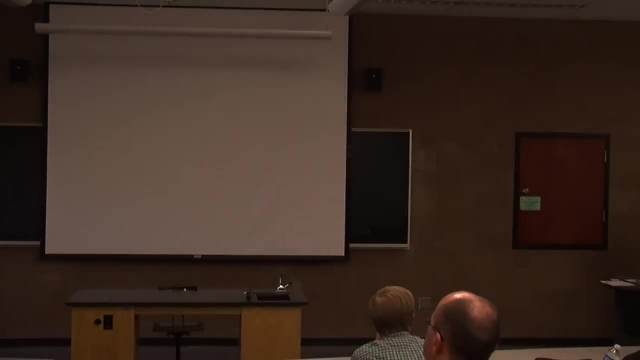 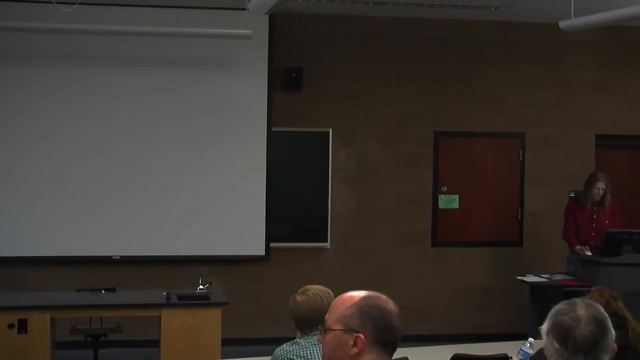 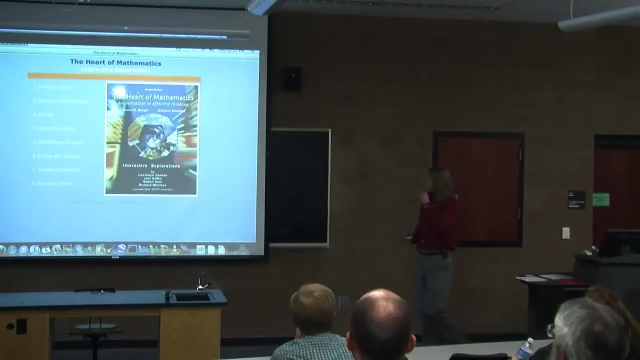 And speaking of zooms in the Mandelbrot set, let me let me pull something up here to show you The liberal arts math class that we teach here. we teach out of this book, The Heart of Mathematics, and this is a disk that accompanies it. 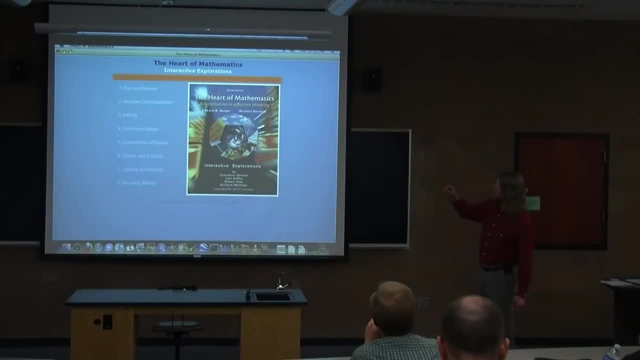 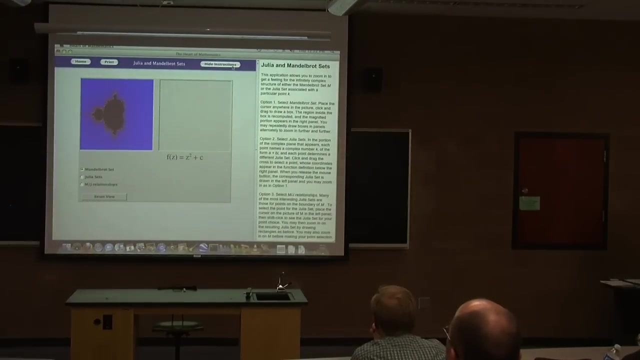 and has a number of really cool demonstrations and interactive explorations. they call them, and one of them is on chaos and fractals. So let me go over here and click on this and notice there's lots of stuff you can do. We're going to look at these sets here. 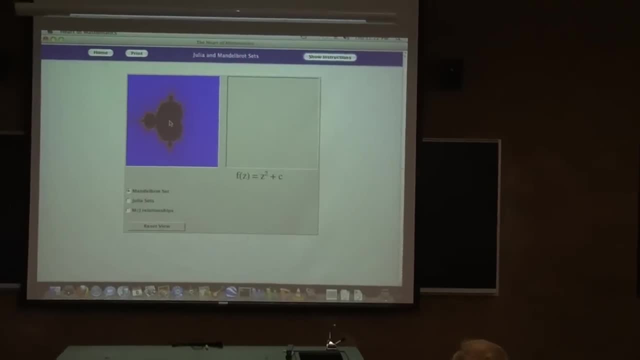 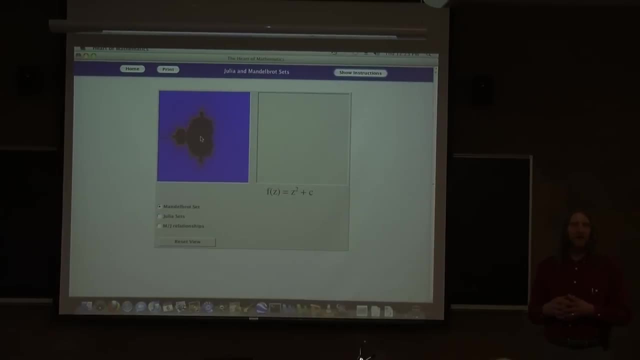 Now this is the standard Mandelbrot set. The thing about fractals is fractals are irregular at all levels of magnification. So you zoom in. so you zoom in to a fractal, it looks kind of jagged and fuzzy. 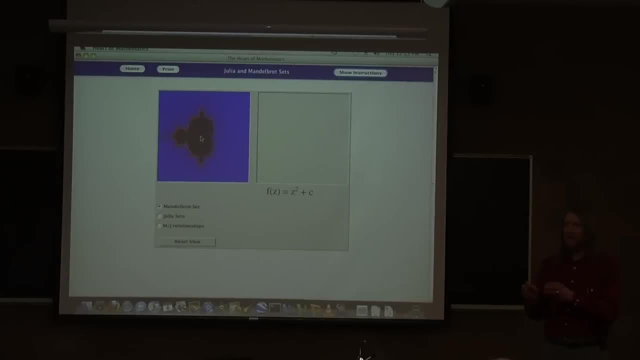 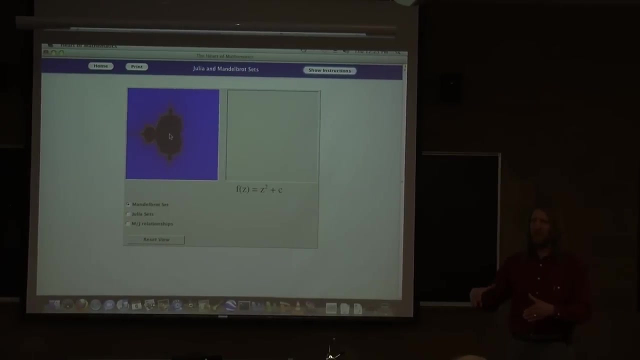 You zoom in, it still looks jagged and fuzzy. You keep zooming in. you can never zoom in to the point where it looks nice and smooth. The problem is if you have a picture of a fractal and you try to zoom in. 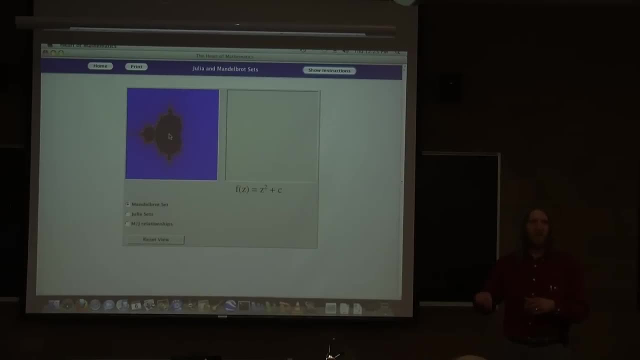 pretty soon you exceed the limits of the resolution of the picture and then it's just a bunch of pixels. So what this little demonstration does is, when you zoom in on a part, it actually redraws that portion of the Mandelbrot set. 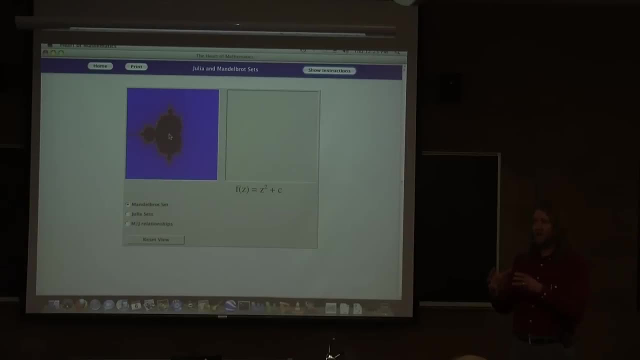 So we're going to zoom in quite a ways here in a minute and we can get around that limitation of photos because it literally redraws that portion of the set when you zoom in. So let's take a look at the area over in here. 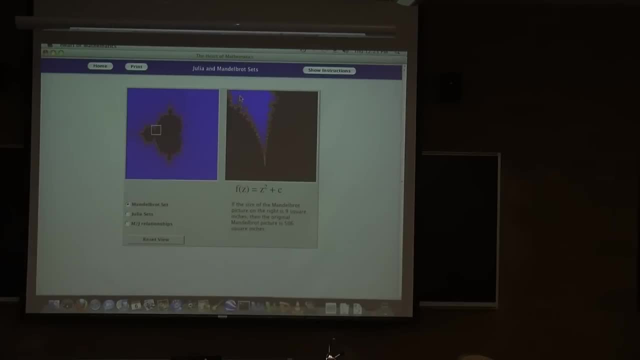 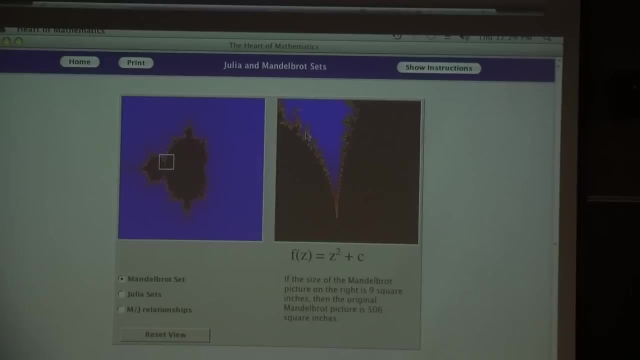 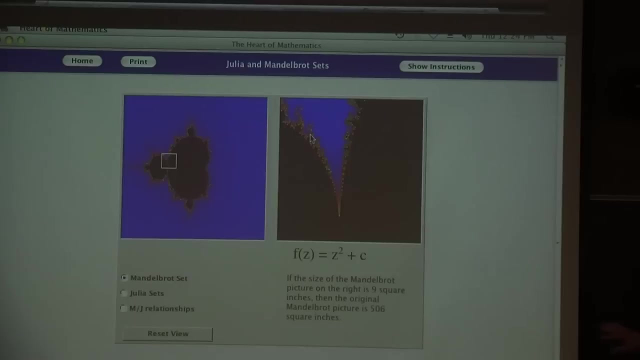 Now, this is known in some circles as the seahorse valley, And if you kind of squint you can sort of see these little guys. they look kind of like seahorses, don't? they? Isn't that cute. Now let me point out to you how this particular demonstration 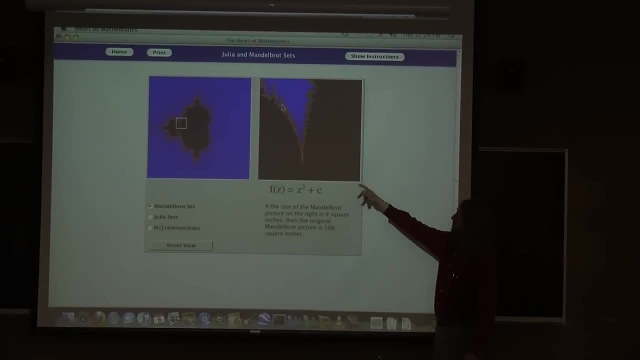 conveys to you the scale When I zoom in. each time I zoom in, the assumption will be that the thing we're looking at is nine square inches. So when I just zoom in a little piece, I zoomed in on if that was nine square inches. 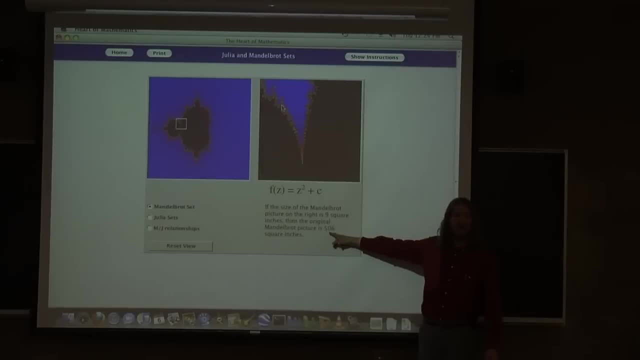 then the original figure must have been 506 square inches. So what's going to happen is this number is going to get bigger as I zoom in, as opposed to telling you how small your viewing window gets. Your viewing window stays fixed and then the original thing we imagine is getting bigger. 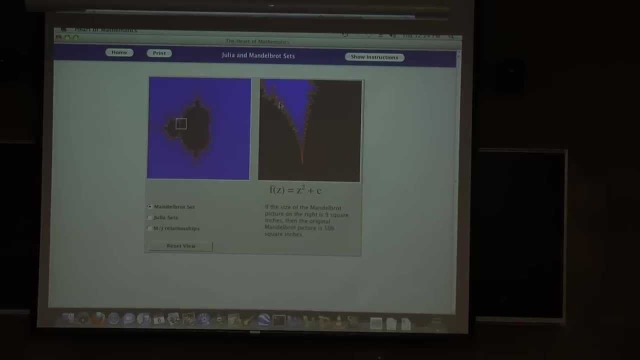 So let's take a look at some of these little seahorse guys in here. That's a little more obvious, isn't it? And you can see that it's still. it's very jagged. you're never going to get to smooth. 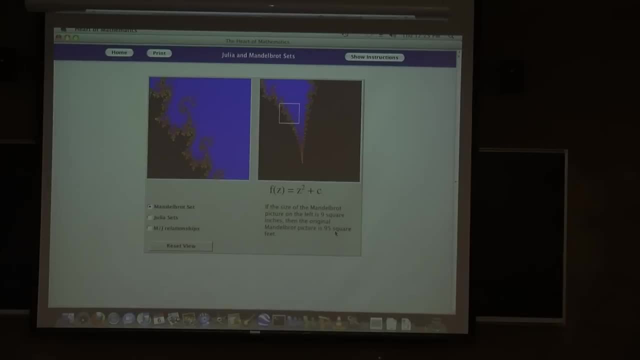 And now, look, now I'm looking at nine square inches out of an original picture that was 95 square feet. Okay, How about let's go in there? Hey, cool stuff. Hey, now, the original must have been 2,789 square feet. 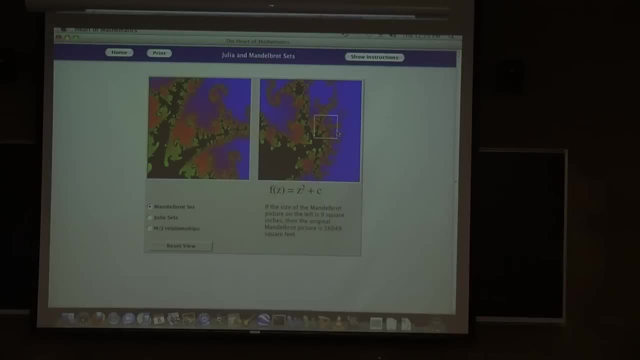 And look, it still looks the same. I mean the same in the sense that it's not smoothing out And you can keep going in, Keep going in, And if you didn't know what level of zoom you were at, there's no way you could tell. 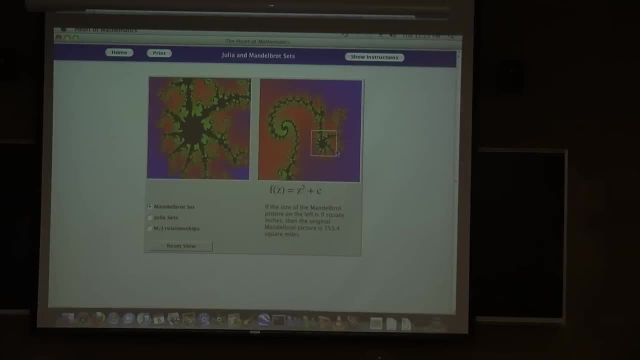 Because the features. there's no sort of periodic repetition, but it still keeps kind of looking the same. Okay, Now look. now we're looking at nine square inches of 26,000 square miles, Okay, And look, it looks sort of like it did to begin with. 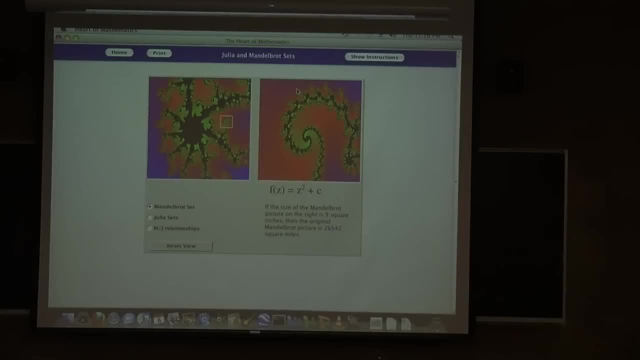 You keep seeing the same sorts of patterns over and over. It never gets smooth. Okay, Zoom in there, Zoom in over here. Now, look, we're up to something like 15 billion square miles. Okay, so we're looking at a nine inch. 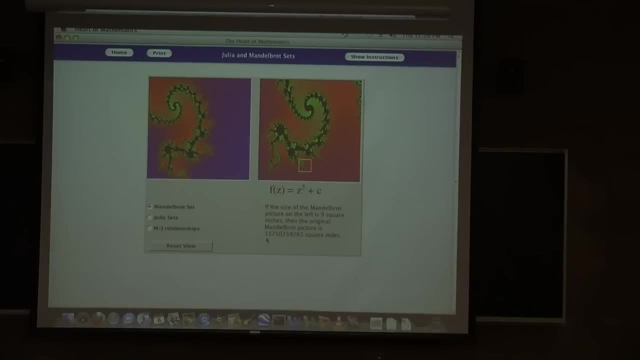 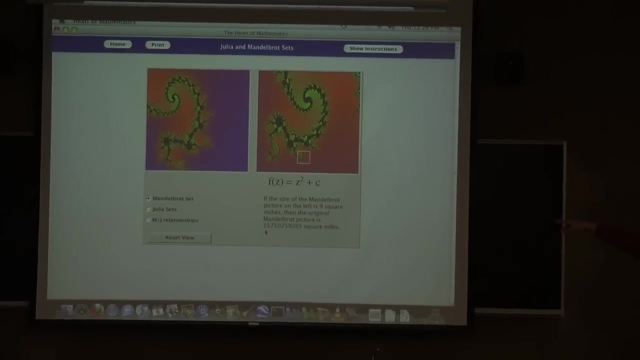 a nine square inch piece of a figure that would- I guess that would easily cover the entire orbit of the Earth. right, Probably even more Okay. so we're looking at just a teeny, teeny slice of this huge thing, and it never gets any smoother. 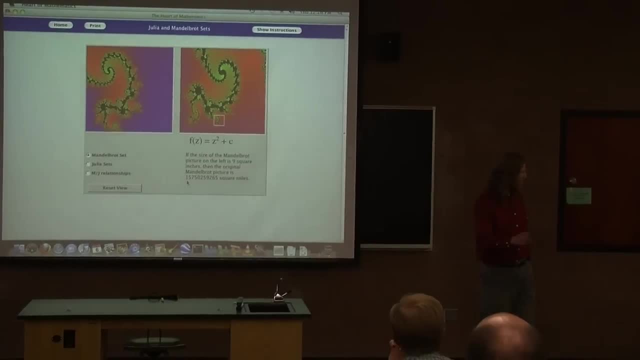 What does this have to do with chaos? Well, remember chaos sensitivity to initial conditions. If you make just a little teeny bit of change in your initial condition, something drastic happens in the long term. Now I don't have the coordinate axes superimposed on this. 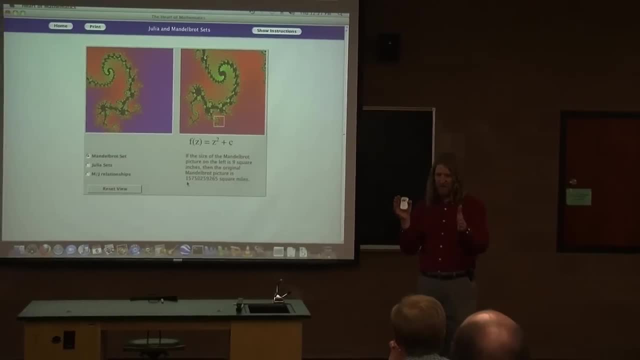 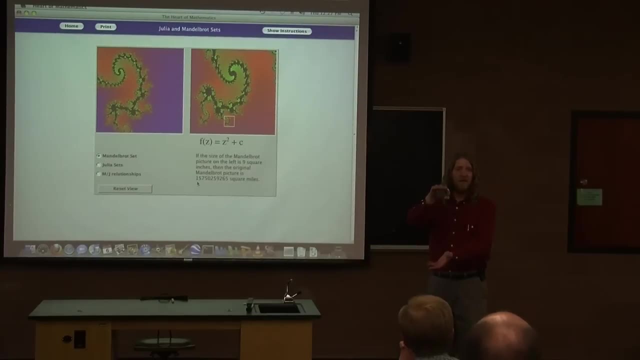 but I will tell you that the original picture that Mandelbrot set lives in minus two to two by minus two to two on the coordinate axes. So it's a four by four box. Okay, Now blow that four by four box up to 15 billion square miles. 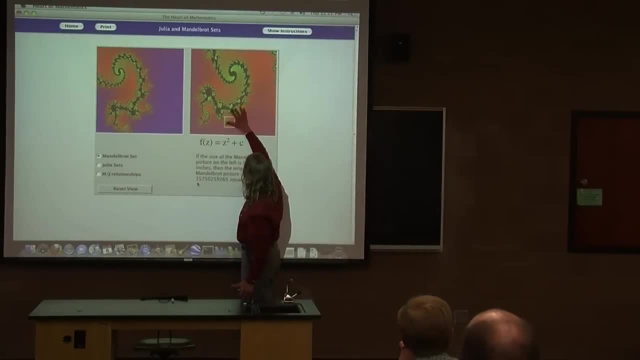 and how close do you think these two points are? Hmm, Not very, Not very. Well now, remember, the original thing was huge and I've zoomed in down to that little teeny spot. Yeah, if I could locate the coordinates of these two points. 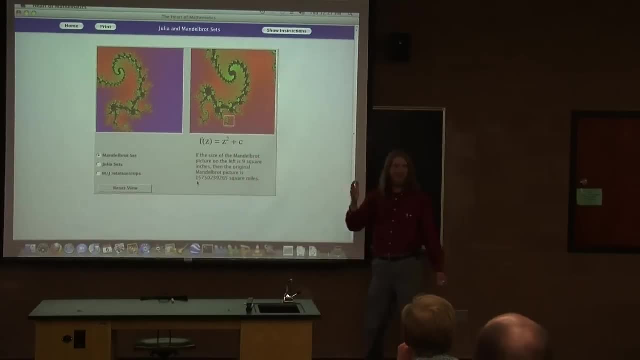 they would probably differ. I don't know. 14th decimal place, But look, one of them stays in the Mandelbrot set. One of them stays close to the origin right, because it's black. it's in the Mandelbrot set. 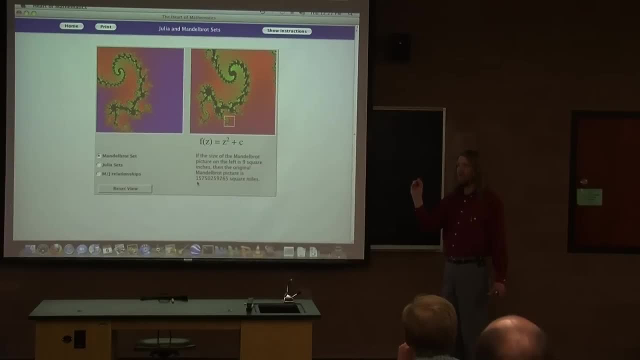 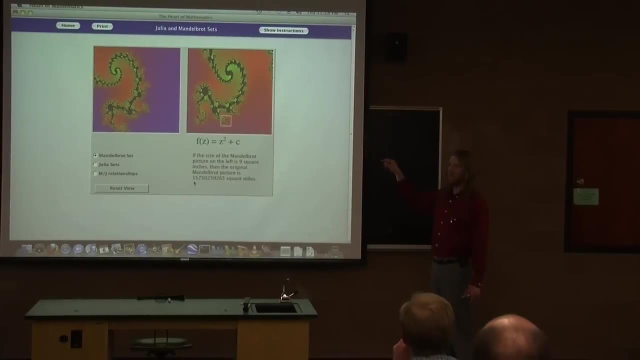 The other one blows up. So that teeny little bit of difference in where you start makes the difference in staying put or blowing up to infinity. That's the connection between chaos and these fractals. This represents infinite complexity. You can never get to a point where you say: 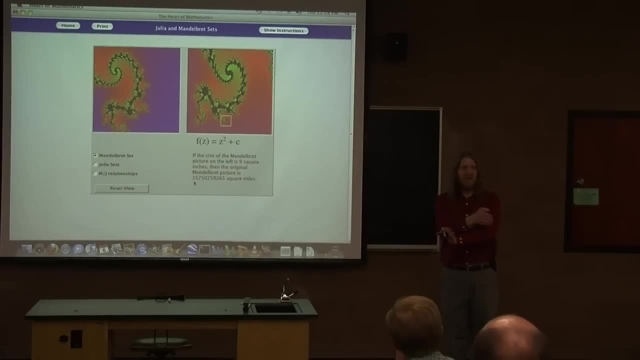 all right, everything here blows up Everything over here, doesn't? Well, no, you can zoom in and be teeny, tiny close. It's interesting to try to break this demonstration. I told you it redraws it and allows us to keep going. 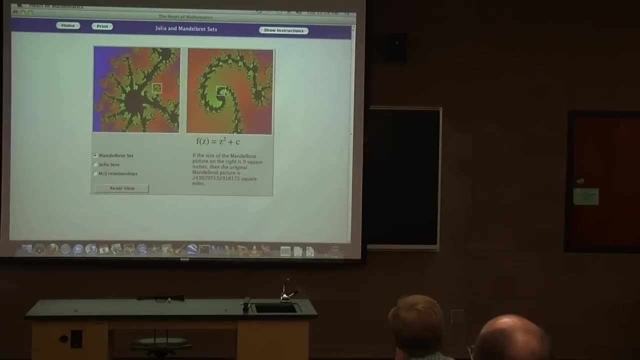 It doesn't go forever. but look at that, Look at this number. How many square lines is that? I don't know, But what happens eventually is the image does get pixelated, And the only thing I can guess there is that it is exceeding. 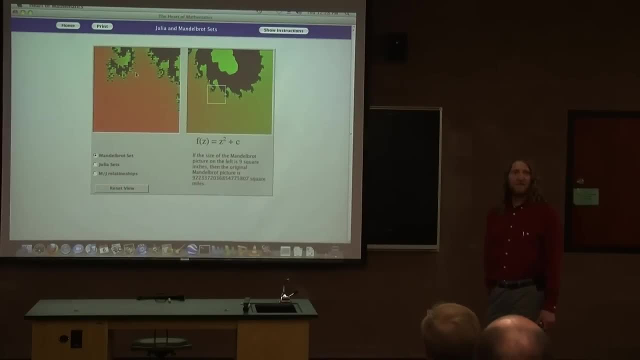 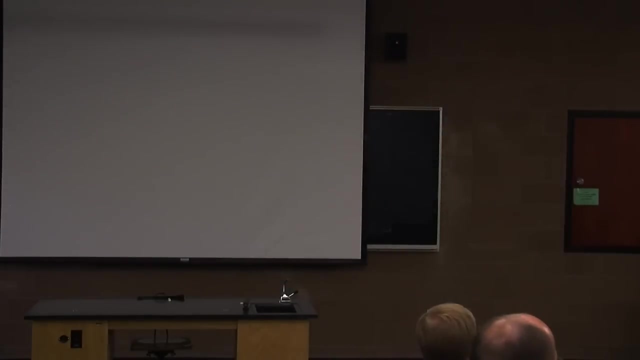 the precision capability of the processor To tell those points apart. Wow, Somebody count that up. No, I'm just kidding. So fractals: Everybody likes cool fractals. I'll show you something else. This is the song and dance portion of the show. 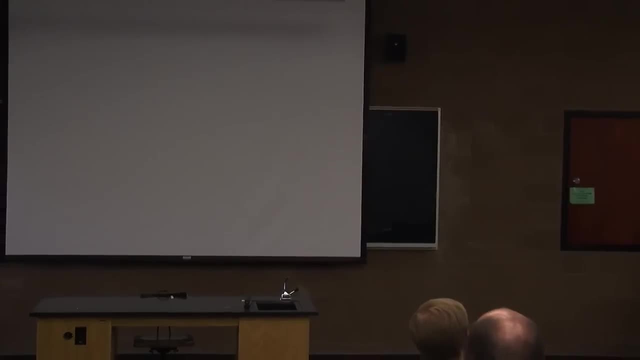 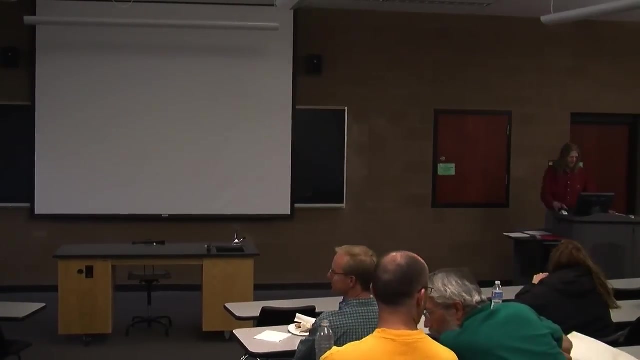 How many of you have heard of Jonathan Coulton? Take a look around folks, Notice it's the computer nerds again. Jonathan Coulton was a software engineer who basically got wealthy enough that he could quit his job and start writing and recording songs. 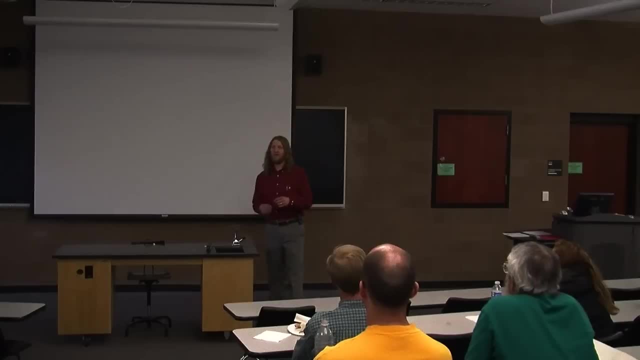 And he did this project called Thing a Week, where he wrote and recorded a new song every week, once a week for an entire year, And they were on all sorts of topics. The most notable probably are his slow ballad rendition of Baby Got Back. 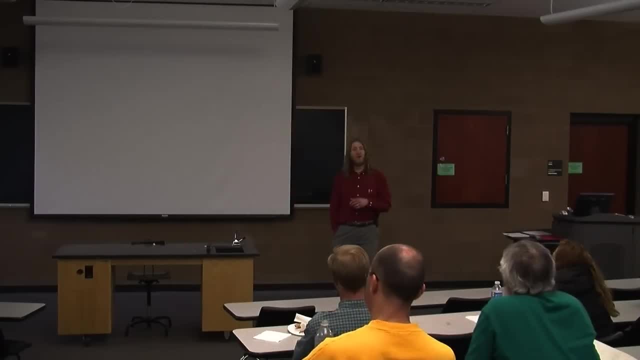 which was kind of interesting. He did one called Code Monkey, which appeals to the computer guys, because that's about his life as a computer programmer. Well, he also wrote a song about the Mandelbrot set, which I'm going to play for you here in a moment. 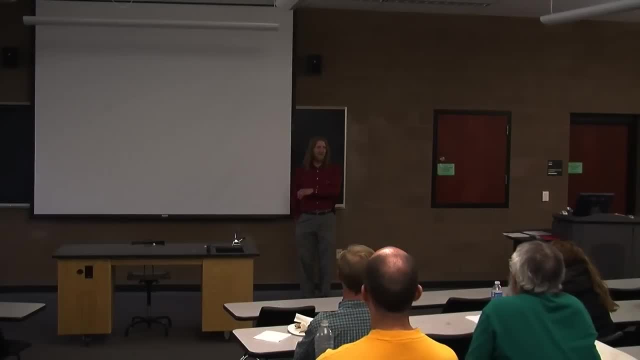 Now he just wrote and recorded these songs, but he's gotten such a big fan base now that his fans have put some of his songs to music, And so what I'm about to show you is some Jonathan Coulton fan took a rendering of the Mandelbrot set. 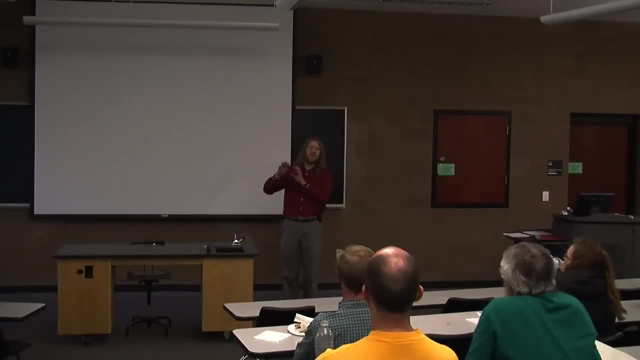 and set to music zooms into the Mandelbrot set. So it's Jonathan Coulton's song. and then somebody made this thing where it's zooming into various parts of the Mandelbrot set And it's rather entertaining. 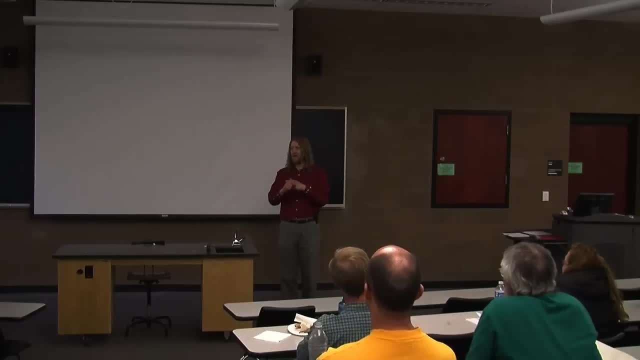 I'm going to tell you two things. One is there are some hiccups in the audio. Okay, Those aren't mine. I've worked and worked and finally figured out that they were in the source file. It seems to me, and I don't know if this is the case. 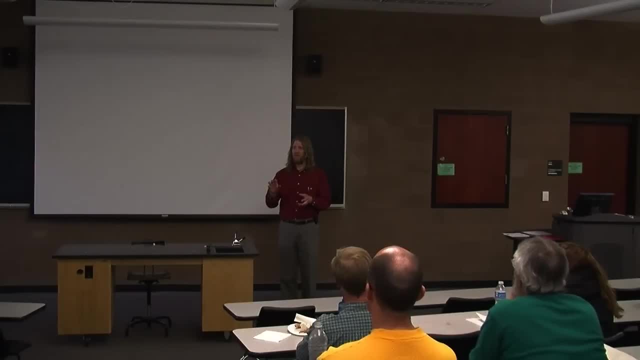 it seems to me like the little hiccups in the audio accompany, the places where the graphics get really intense, And so I'm guessing that the person who encoded this, that their processor, had problems at this point. Okay, So I apologize for that. 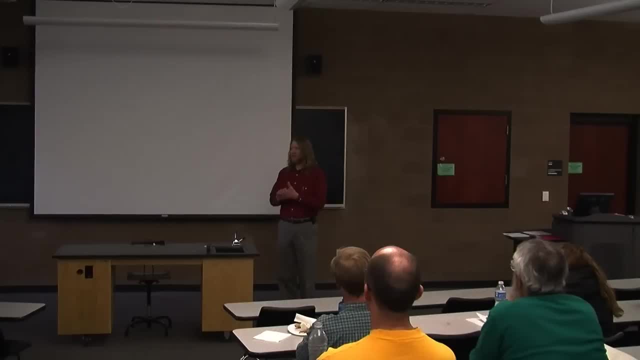 The second thing I have to tell you is that if you have delicate sensibilities- there are some, well, there's some language in the song that might offend you, And if that is the case, then you should perhaps close your ears or leave. 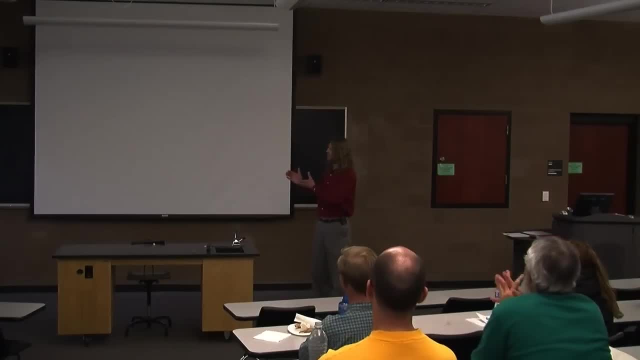 Again, it's not my fault, It's Jonathan Coulton. But I would not. I wouldn't pretend to be offended by it myself because I don't think it's funny, But I wouldn't want to destroy the artistic integrity of his work by attempting to censor it. 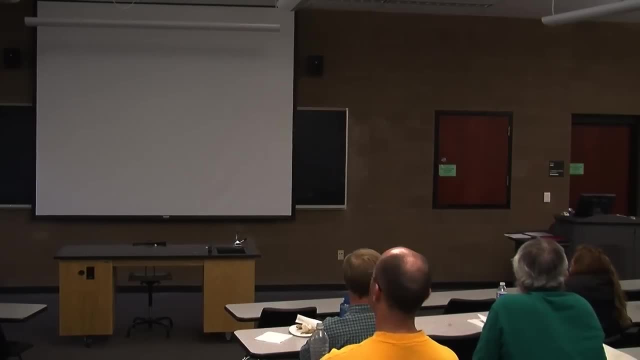 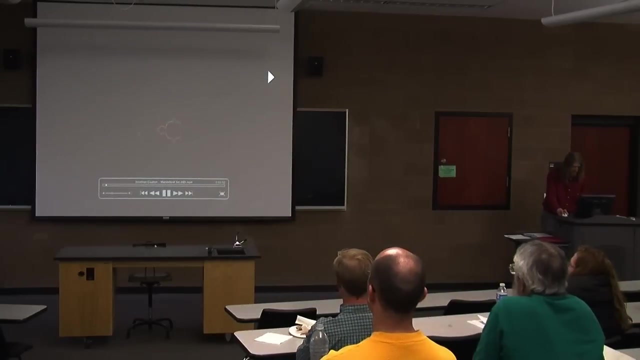 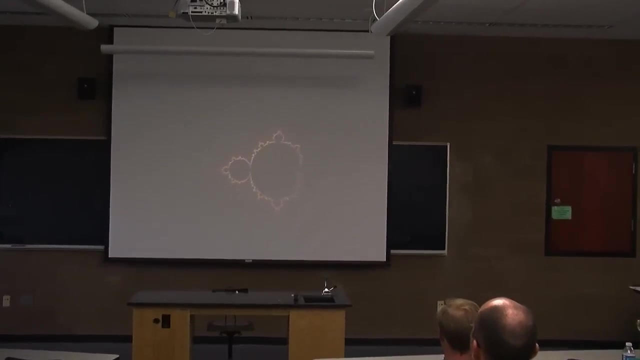 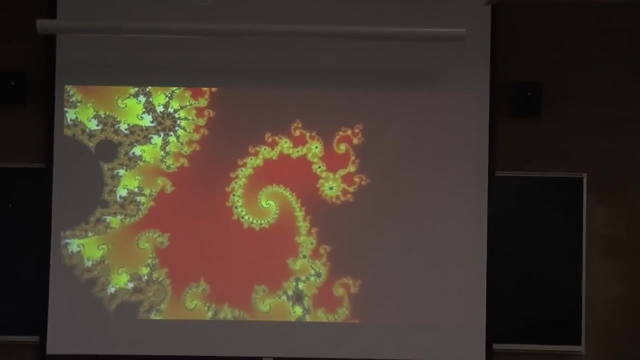 So Let's see, Everybody see, that There's no one prone to seizures in here. They're like flashing and Right, okay, And then there's the cat. You know him, right, Right, That's the cat, There's the cat. 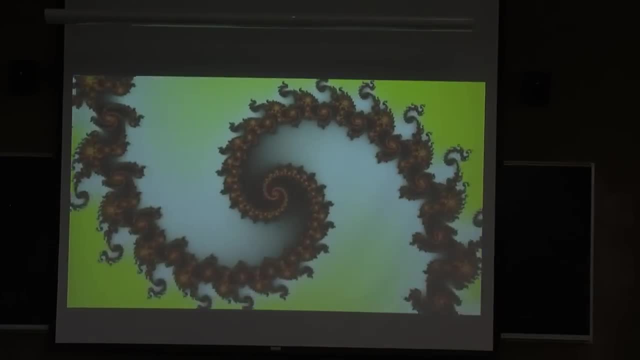 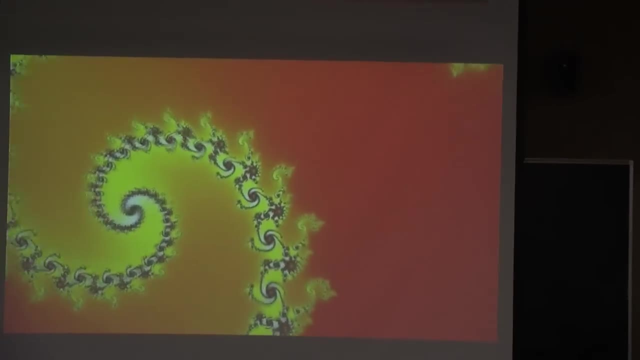 Can you guys hear it? Yeah, Yeah, Yeah, Listen to this. Oh, oh, yeah, Yeah, The cat's RIP To all of you out there. He's just been in this life for a long time. He can't quite get saved. 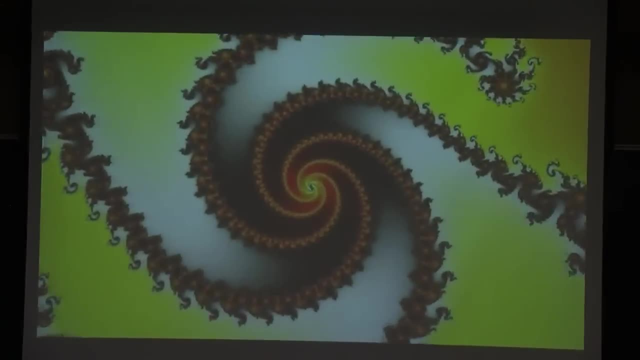 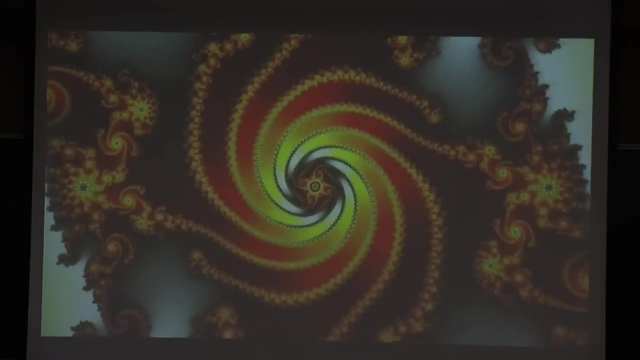 Dude, he could be standing up right now. Oh, he can't. Oh, you're not. Yeah, Yeah, Yeah, So, um, Uh, There's something in there. I've got a plan that's way longer than the day. 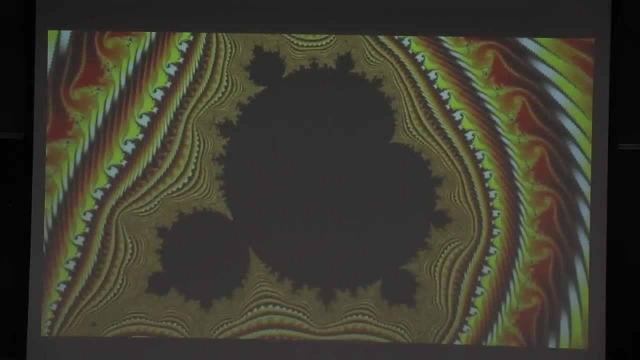 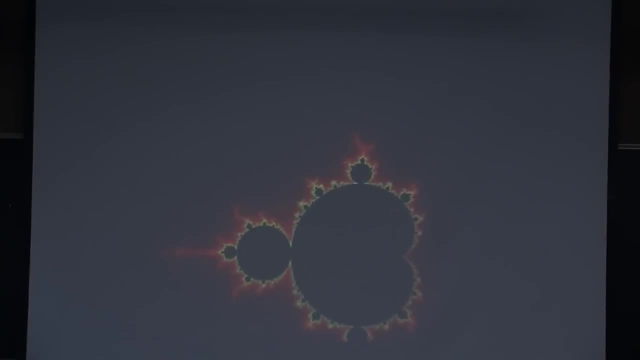 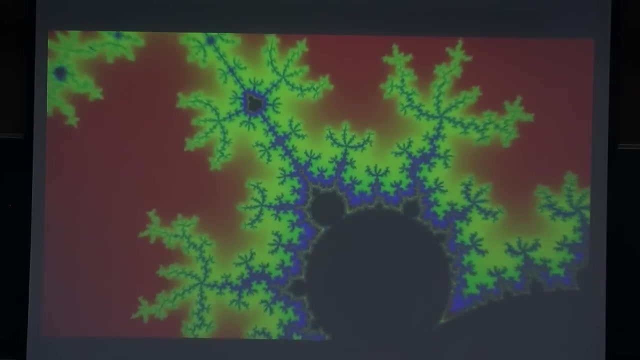 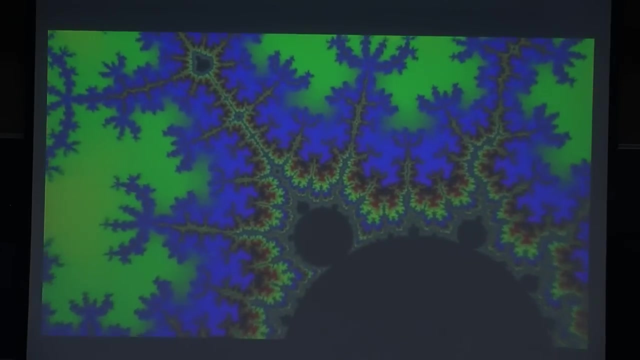 A man named Benoit, man of rock and war With the state of your mathematics And his unique geomagical insights, Left him well equipped to face those demons down. He saw that infinite complexity Could be described by simple rules. He used his giant brain and he turned the game around. 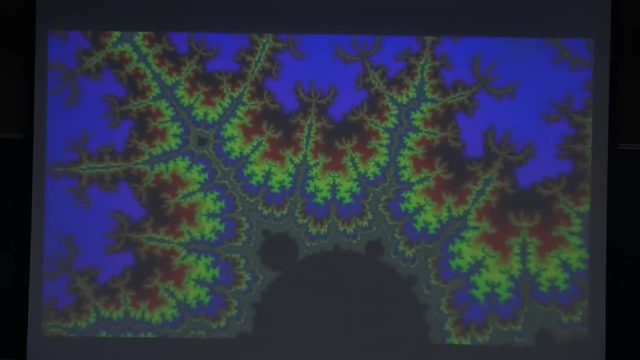 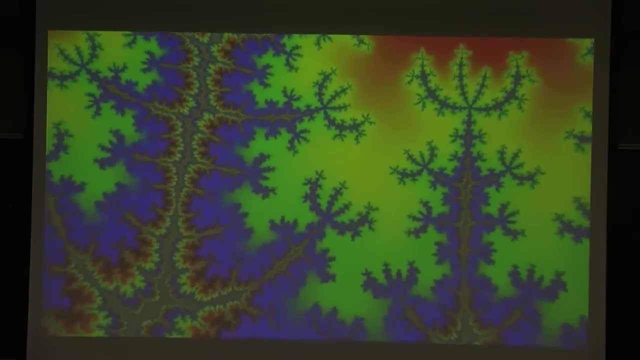 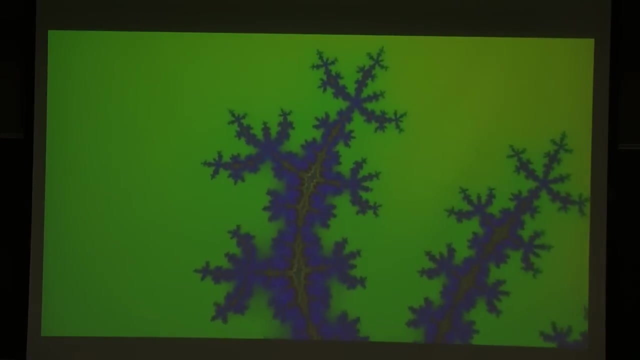 And Benoit was the star, The star of religion and the set Of all those points in the form, Picked his pencil up and wrote his secret down. And Benoit was the man of rock and war And his unique geomagical insights Made a point called C in a complex plane. 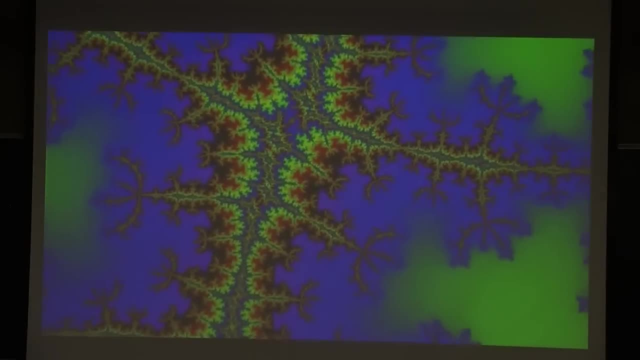 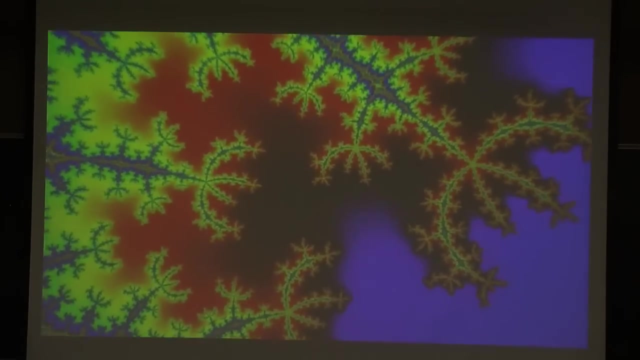 Z1, B2, square plus C, Z2, Z1, square plus C, Z3, Z2, square plus C. And he saw that the series of C's will always stay Close to C and never trend away. That point is in the man of rock's head. 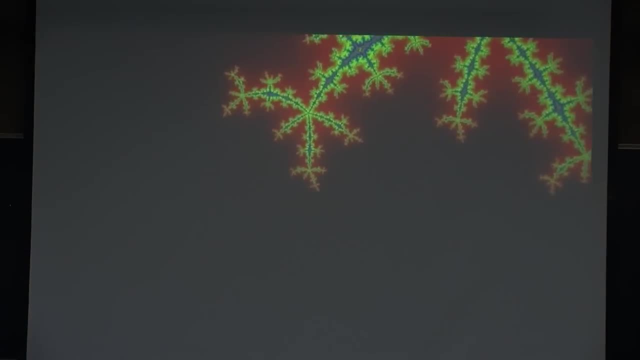 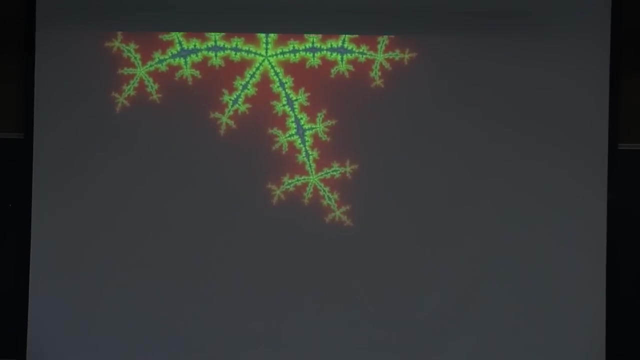 Man of rock's head. You're a shock test on fire, A day of pterodactyl. You're a heart-shaped box of springs and wire. You're a heart-shaped box of springs and wire. You're one bad-ass buggy racked up And you're just the time to save the day. 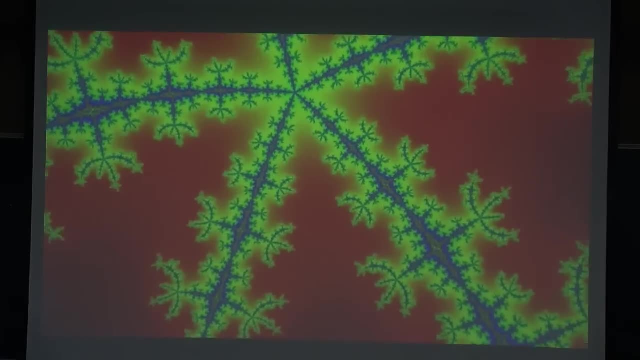 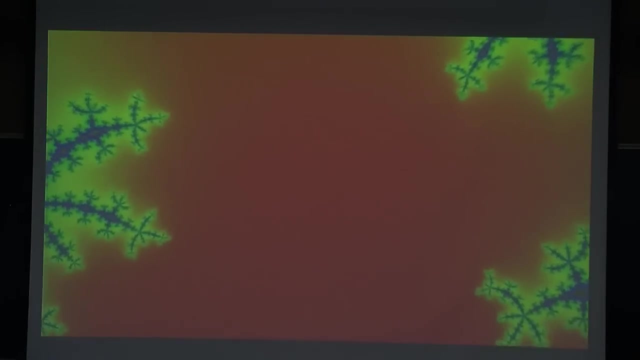 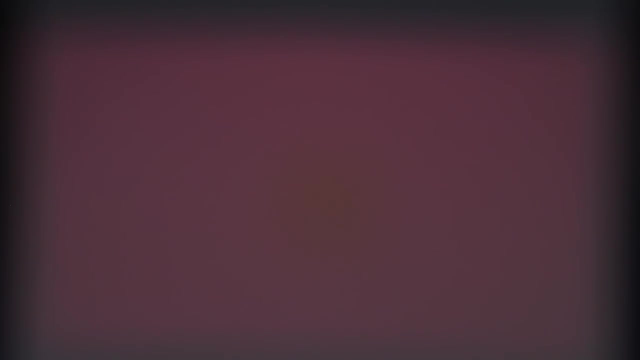 So give it up. here's your way. You can change the world in a tiny way. Man of rock's in heaven, At least he will be when he's dead And I'm still alive. and teaching math. and gale Gave us order out of chaos. 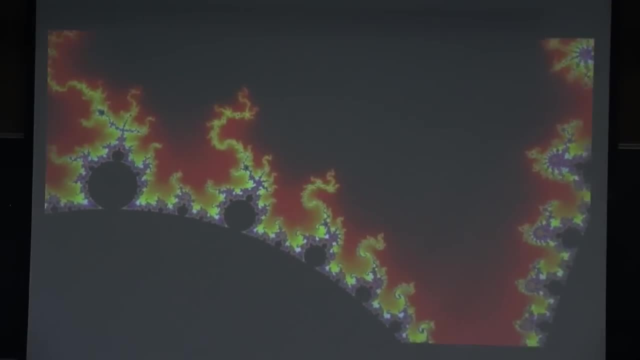 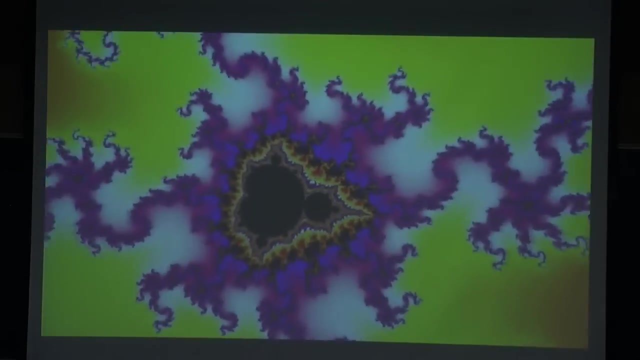 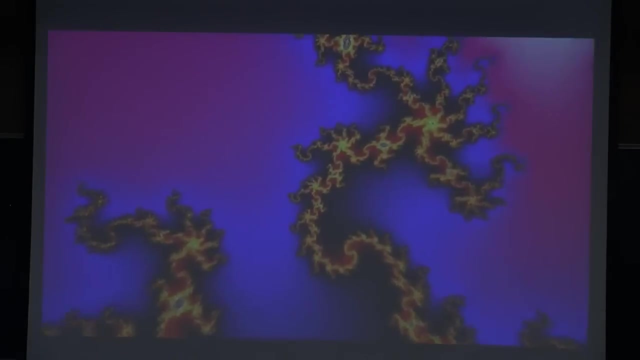 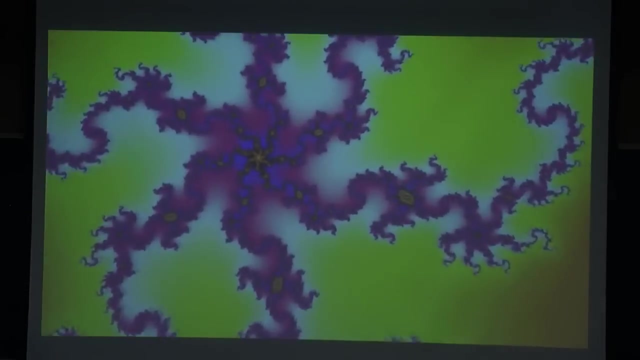 Gave us hope when there was none, And geometry succeeds where others fail. If you ever lose your way, But a fly will flap its wings From a million miles away, A little miracle will come to take you home. Just take a point called C in a complex plane. 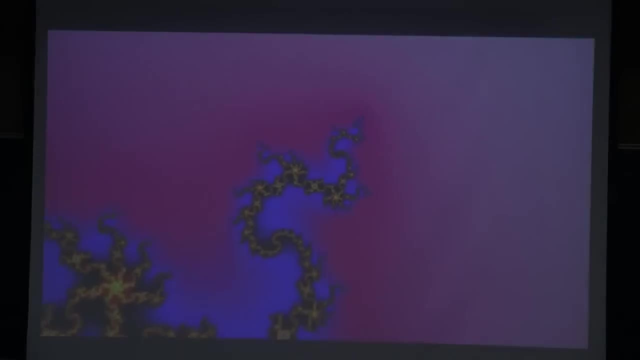 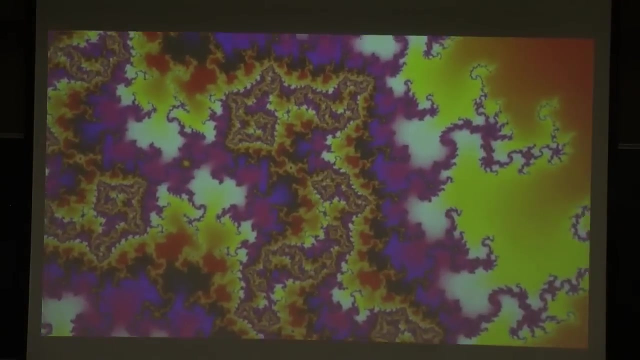 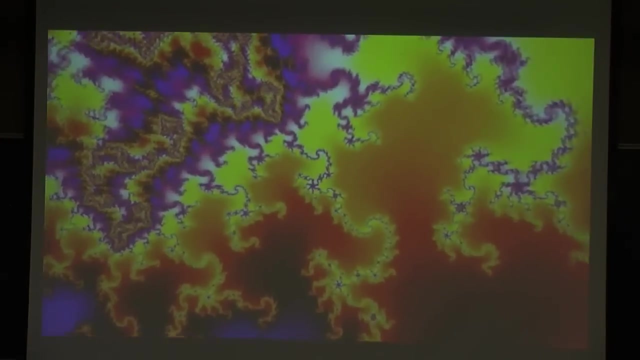 Z will be the square for C, Z2 is equal to square for C, Z3 is equal to square for C, And so the series of Z's will always stay Close to Z and never trend away. That point is in the man of rock's head. Man of rock's head. 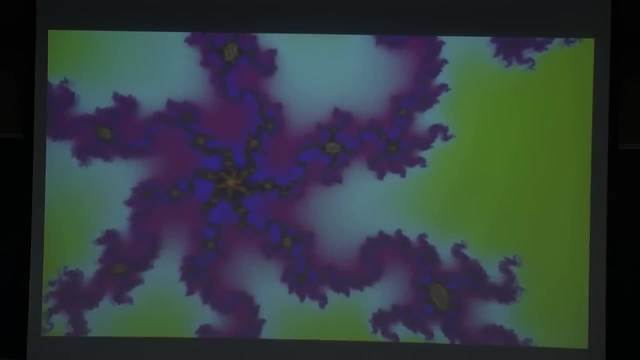 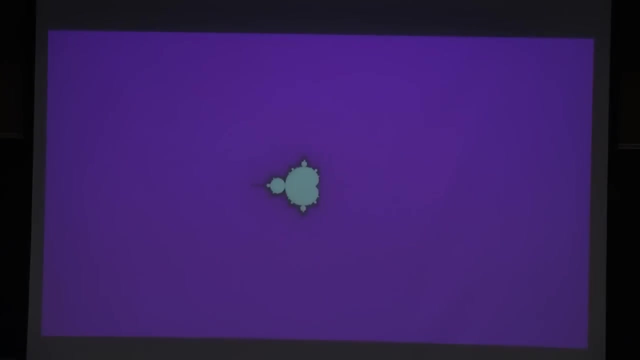 You're a shock test on fire, A day of pterodactyl. You're a heart-shaped box of springs and wire. You're one bad-ass buggy racked up And you're just the time to save the day. Sweep it all out of fear's awake. 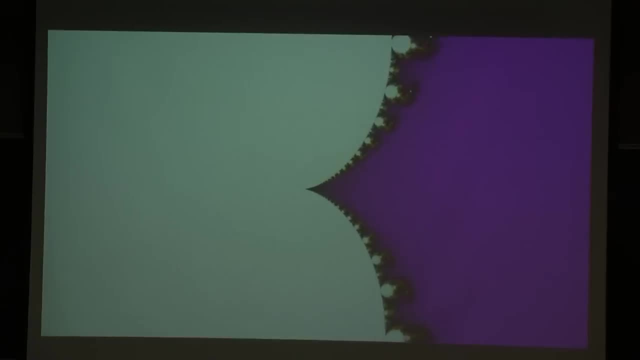 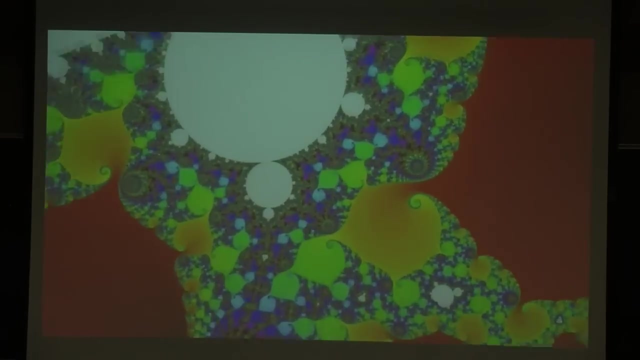 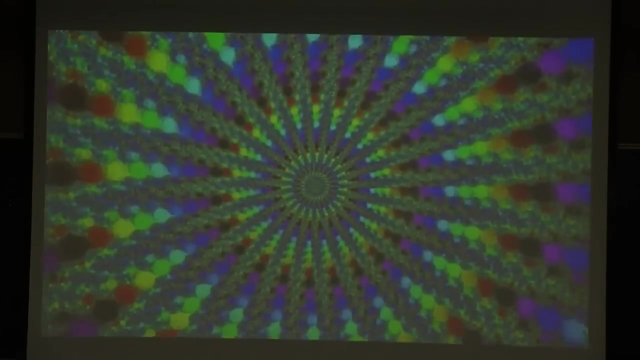 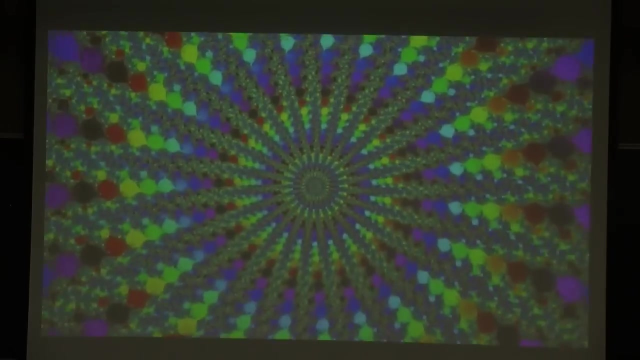 You can change the world in a tiny way And you're just the time to save the day, Sweep it all out of fear's awake. You can change the world in a tiny way. A-won't change the world in a tiny way. A-won't change the world in a tiny way. 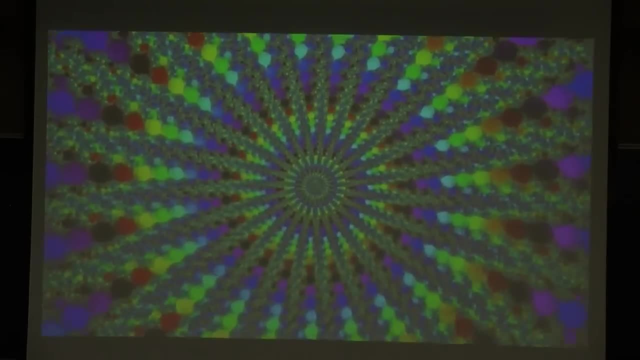 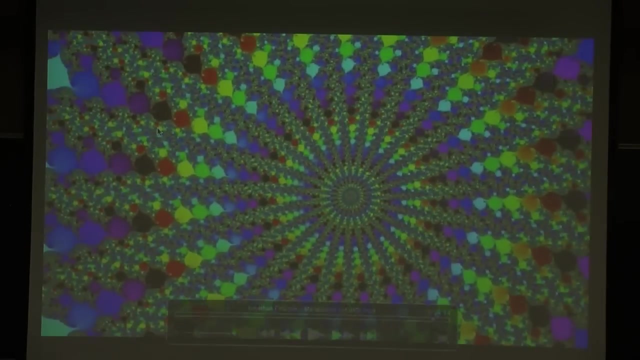 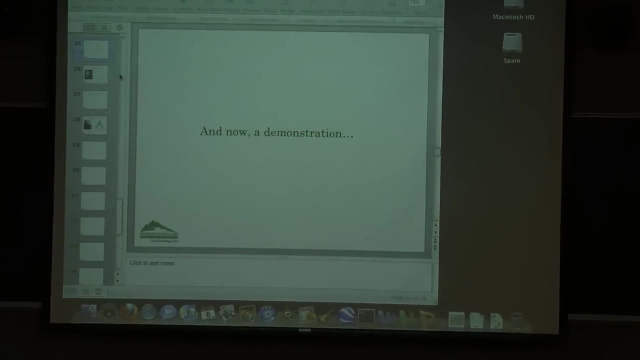 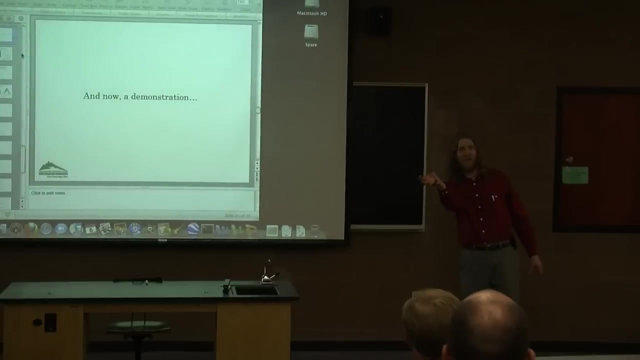 Cool huh. Did you notice how many places that kept zooming in and zooming in and you kept seeing another exact copy of the original Land? O'Rourke set the little snowman on his side there. That's just amazing, I think. 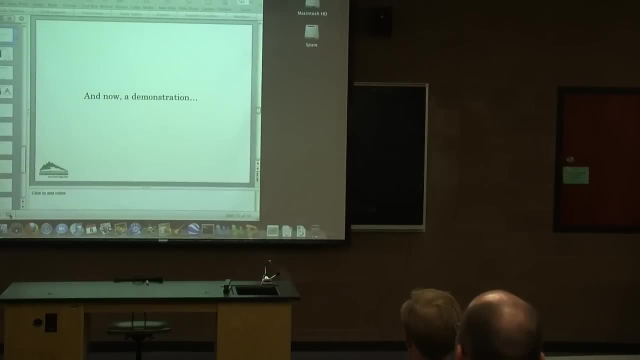 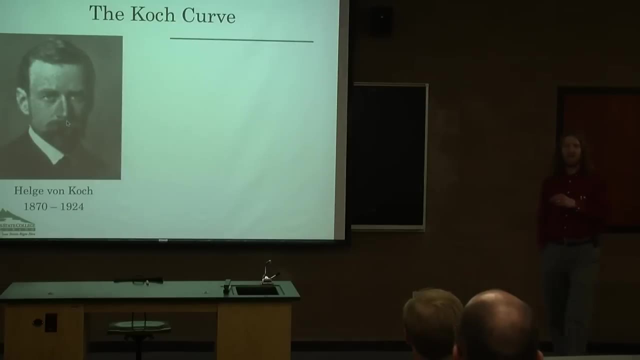 and so do many other people. Now let's talk a little bit about what he said in the song, because he mentioned a couple of things that I have not yet talked about. He talked about the Koch curve. okay, The Koch curve is named after. 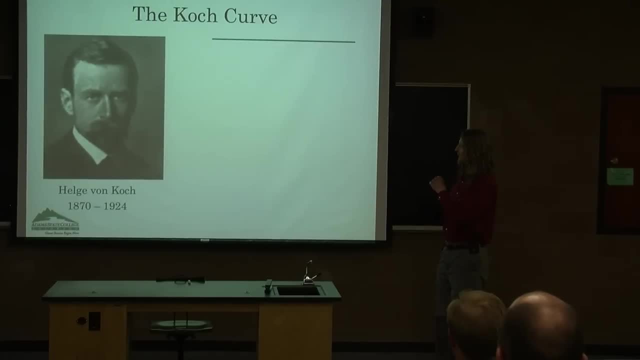 Swedish mathematician Helge von Koch, and he started with a very simple line segment like this. So here's the construction of the Koch curve: Start with a line segment and then cut out the middle third of the line segment and then cut out the middle third. 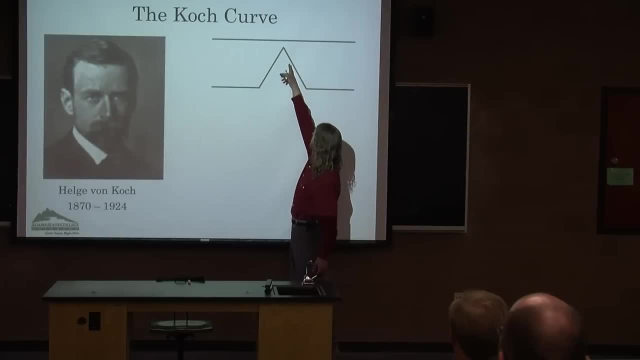 and then cut out the middle, third, and then patch in two pieces that are the same length in there. Another way to think about this is you can think about cutting right here, bending that piece up and then sticking another one in there, like that. 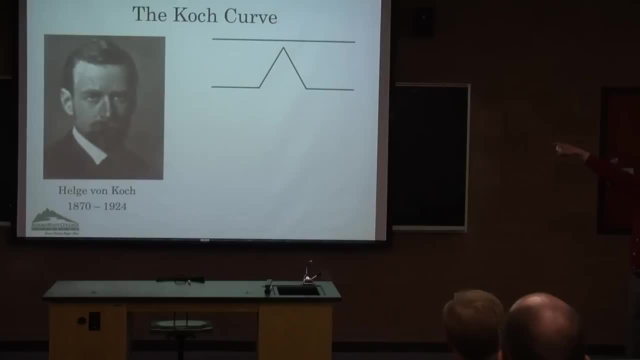 Now, if the original segment had length one, you can figure out pretty quickly that this one has length four thirds. okay, Now you repeat this process on each of the remaining little straight pieces there and you get a picture like this and you can figure. 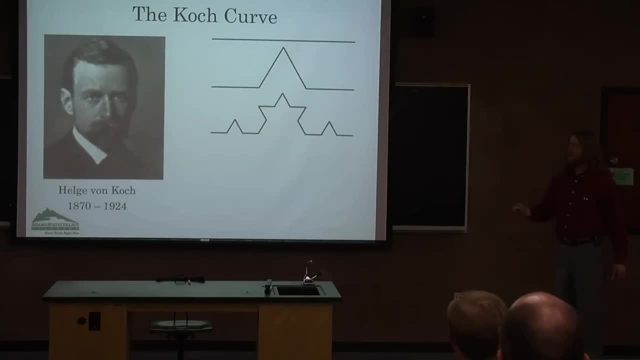 that its length is four thirds squared. Do it again. this thing has length four thirds cubed, and four thirds to the fourth, and so on and so on. You keep doing this. what you wind up constructing is a curve that has infinite length. 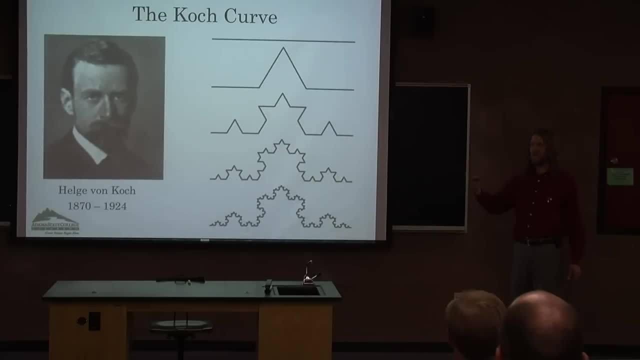 Right, Four thirds is bigger than one, and we've already seen that if you take something bigger than one, well, we just squared it over and over, but it still works if you just raise it to the third power, fourth power, Fifth power, sixth power. 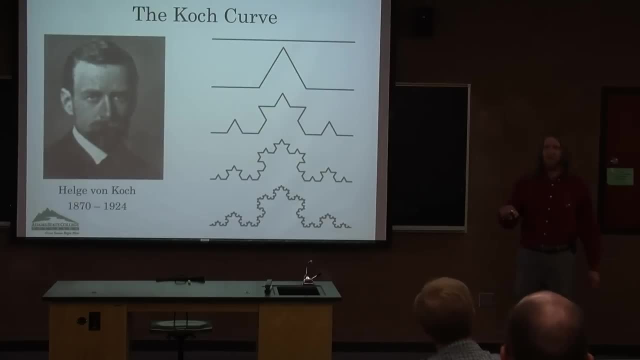 So the ultimate result of this has infinite length. Well, maybe It also for those of you who know the lingo of calculus. it's also nowhere differentiable. It is continuous, but nowhere differentiable. It is so jagged it is infinitely jagged. 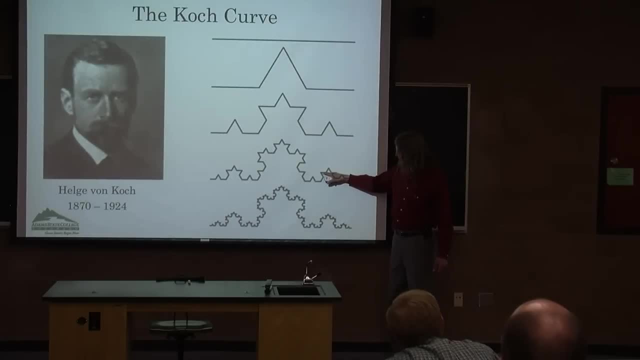 You cannot zoom in and zoom in until you get to a point where there's a little straight piece, because there aren't any, It is infinitely jagged. and when you get to a situation like that, well, you can sort of have a philosophical discussion. 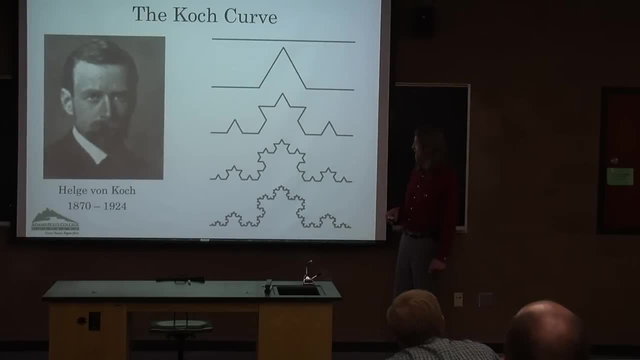 about what does length mean? anyway, The other thing that happens- and I don't have time to show you why this works, but the other thing that happens- is it goes from being: well, this was one-dimensional, right, This really is still one-dimensional. 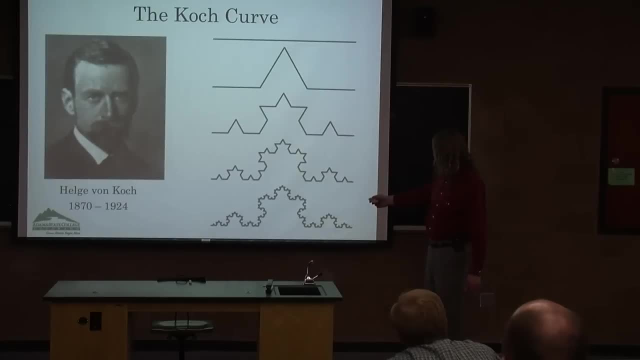 because it's a bunch of one-dimensional pieces stuck together. What happens in the limit is this thing turns out to have dimension well greater than one, but smaller than two. It's, you know, I don't know. It's somewhere in between one- and two-dimensional. 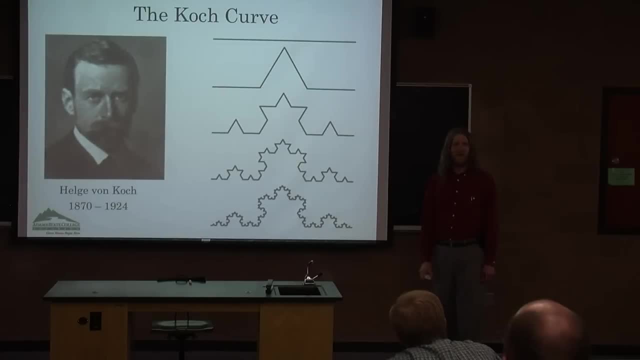 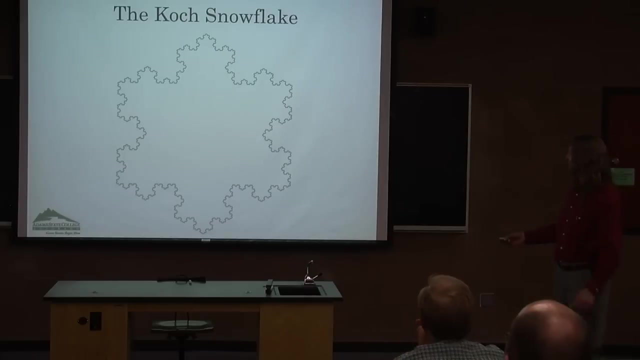 and I've never really understood it either. It's weird, But, as John Conway once suggested, in math you don't really understand things, you just get used to them. So I'm kind of used to it by now. You'll often see this done in a slightly different way. 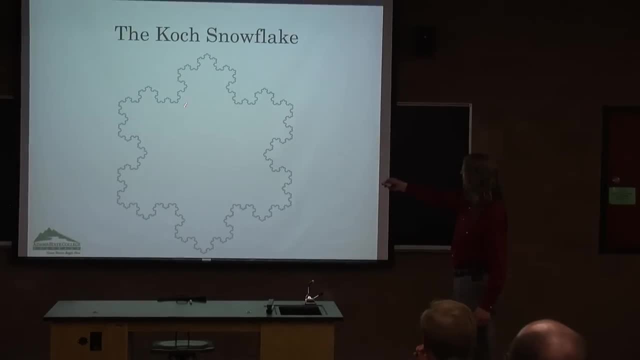 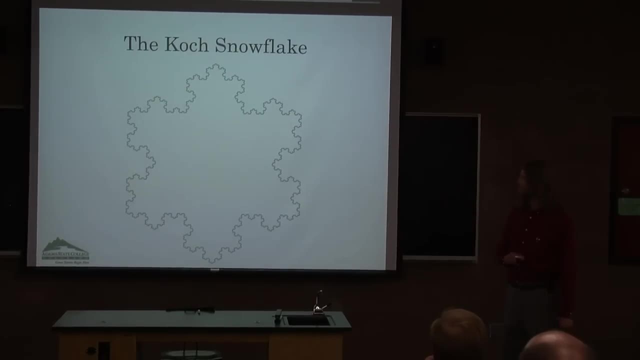 Instead of starting with a single line segment. if you started with an equilateral triangle and did that construction on each side, you get this thing called the Koch snowflake, which also has infinite length, but of course it encloses a finite area in an infinite perimeter. 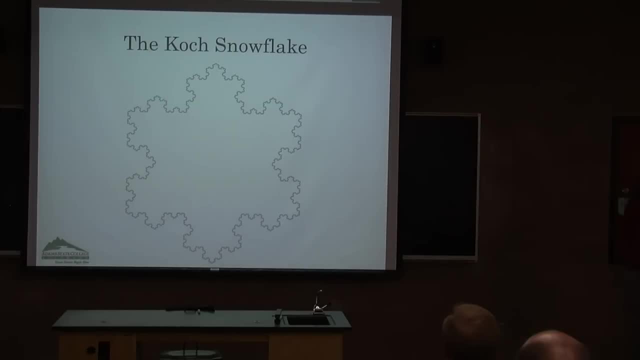 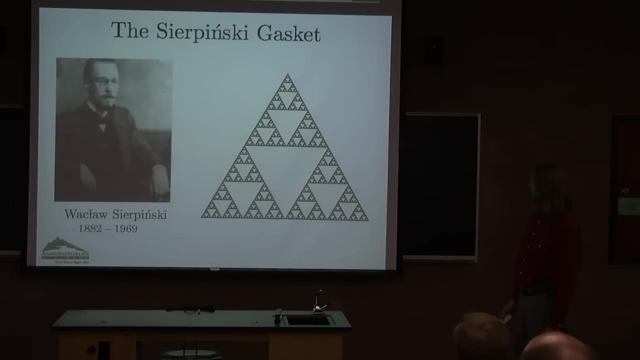 Okay, Interesting. He also talked about the Sierpinski gasket, and the Sierpinski gasket is another fractal named after this guy, and I would not even pretend to know how to pronounce that first name, because it's Polish. 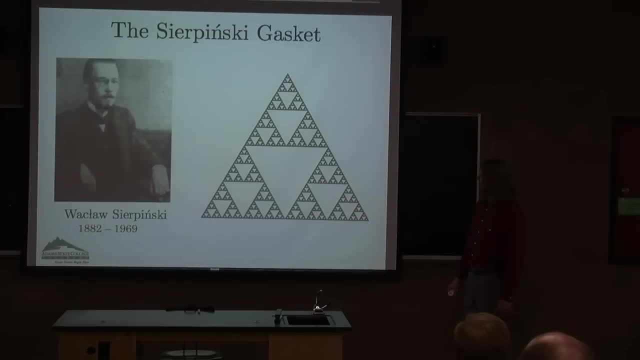 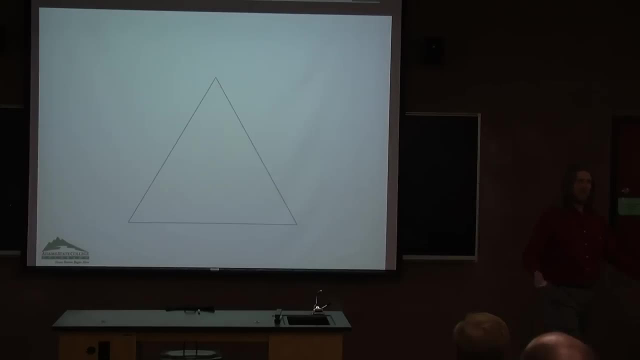 and the last one's, Sierpinski. I can do that, okay. Now this is sort of the end result. How is the Sierpinski gasket formed? Well, if you do a triangle, start with an equilateral triangle like that. 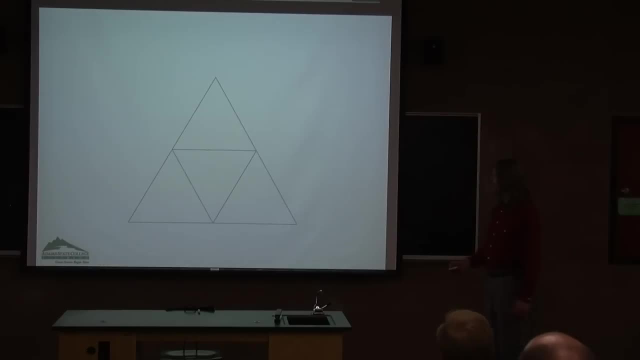 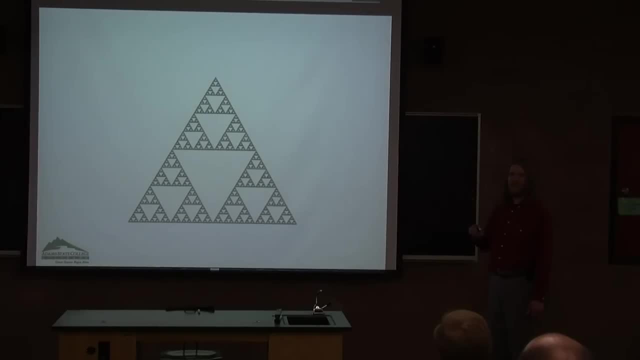 those lengths add up to well, infinity, and at this point it's really not even appropriate to say little segments, because this has that same property: that, in the limit, the thing that you wind up with has swollen up out of one dimension. 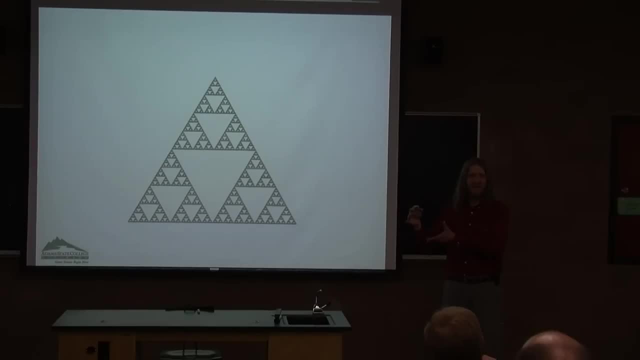 It's now also between one-dimensional and two-dimensional, so you couldn't really find any segments in there, because that would mean that I don't know what did it swell up? Did it get Got waterlogged or something? I don't know what happened, but it's pretty interesting stuff. 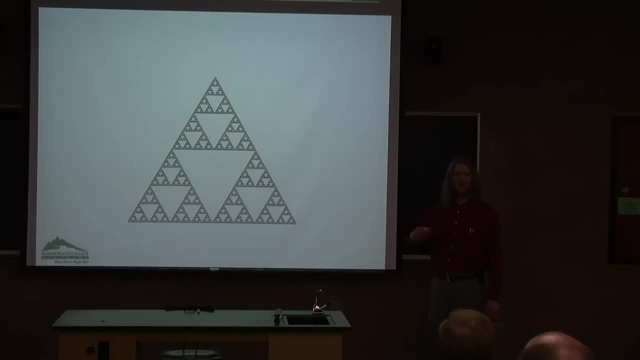 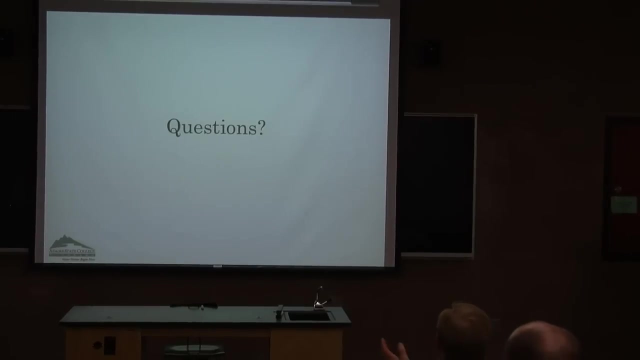 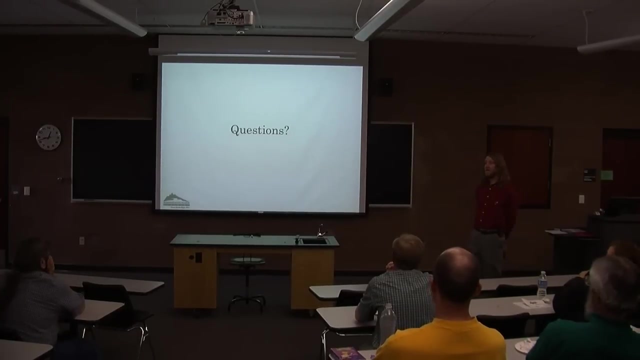 There's also several varieties of this, depending on whether you start with a square or a triangle, and you can do three-dimensional versions of these and probably higher-dimensional. but what questions do you have now? Any questions? Yes, You used the word intense a few times. 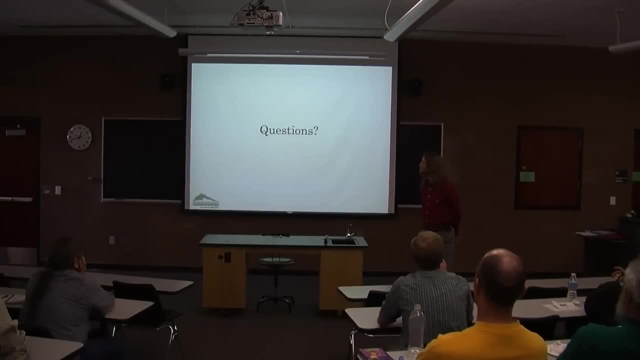 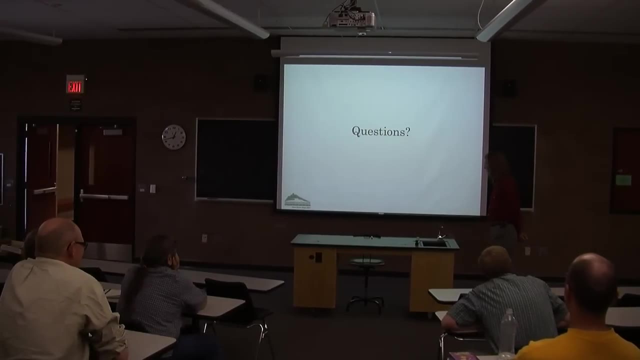 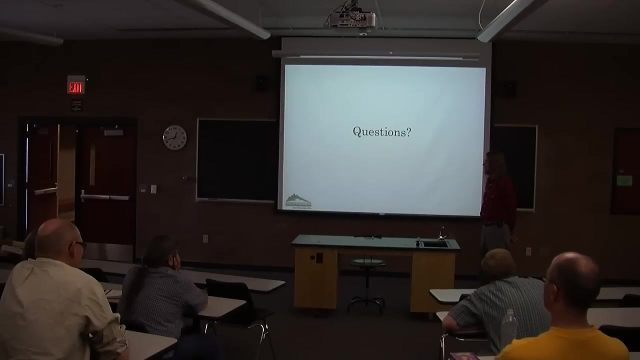 Is that a technical term? Hmm, I don't know, but I'll make it one if you like. Sure, I would use it Where there's more density of patterns and more space, or Well, I was using it sort of an eyeballing the picture. 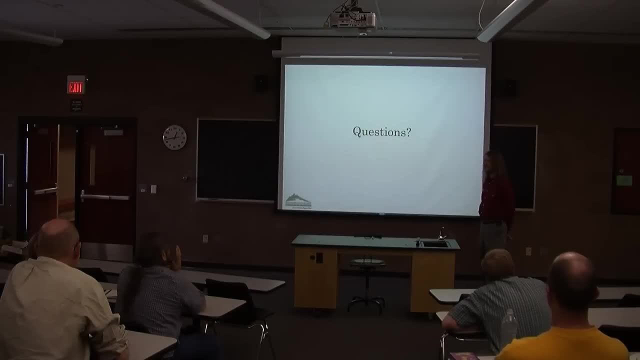 a pretty picture. The thing about the sets that Amanda brought, said, is you couldn't really say that any portion of it was any more intense than another, because there's this infinite complexity. You can't get to a point where, oh okay, now we've got big polka dots. 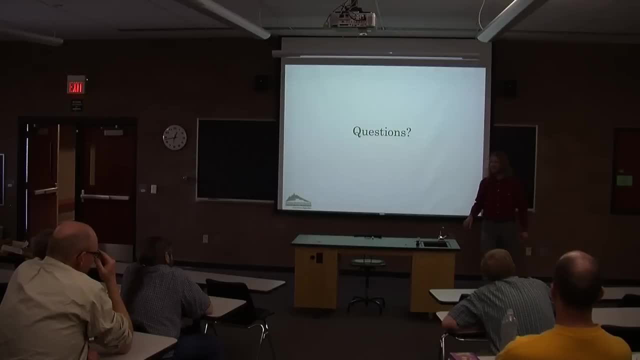 and everything's. you know it's always got these little jagged pieces in there, But just from a visual standpoint, as far as rendering the graphics, I think that more let's see I'll have to go back to that. 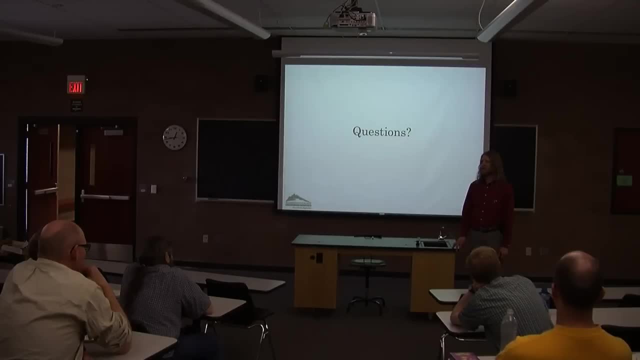 I'll have to go back to that. I'll have to go back to that. I'll have to. I'll have to write down a, a rigorous definition of that, But it would have something to do with the number of pixels of different colors located in a certain area. I think is what I'm coming to. 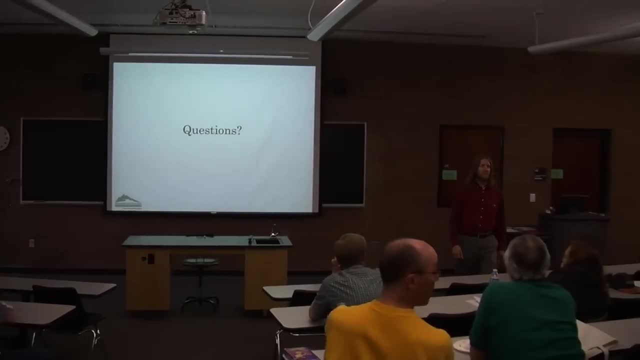 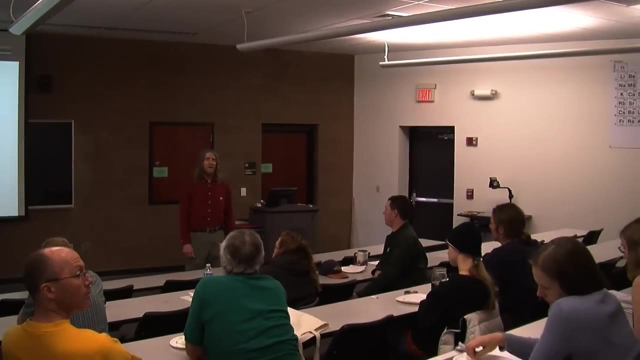 Yes, You mentioned that used a computer graphics program to generate these images. Do you know what that was And if it's obviously it's changed now and in this time, and what we use now to do that? Actually, from what I understand, 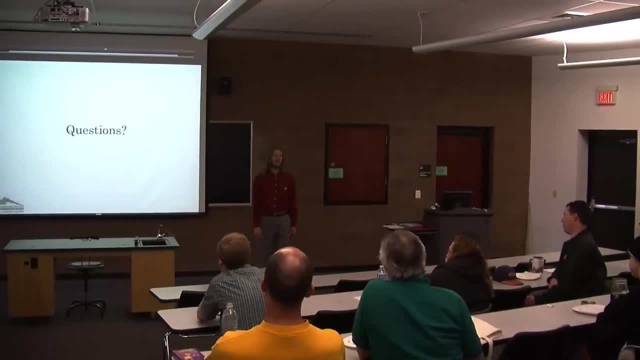 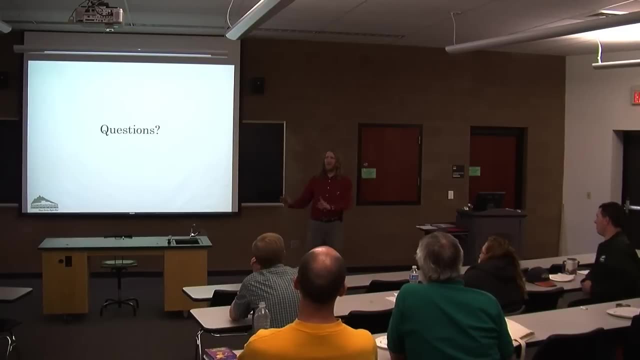 he had to write that himself Because the computer graphics in the in the day 1970 were, it's kind of like, the old green screen monitors- I don't know if any of you are old enough to remember those- So he had to. he had to write the program not only. 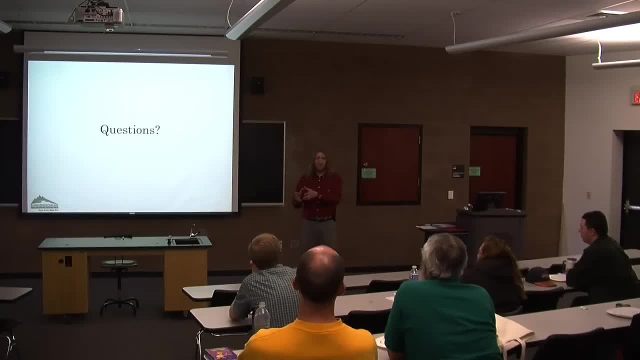 that would render the Mandelbrot set, but he had to write the program that would draw a picture of it on the screen, And so I. that's all I knew about that. Yeah, that Mandelbrot originally started his work. 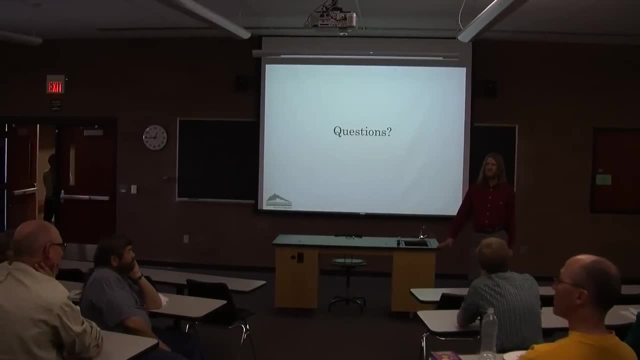 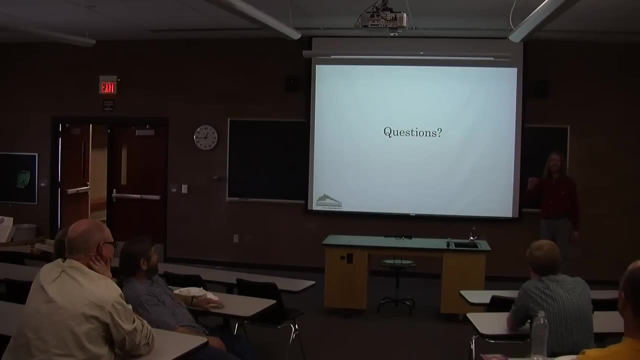 at some French university and quit because they were too constricted in their thinking there. Yes, Well, you may have heard the line in the song of his disdain for pure mathematics. He didn't really care for pure math, wanted to do applied stuff. 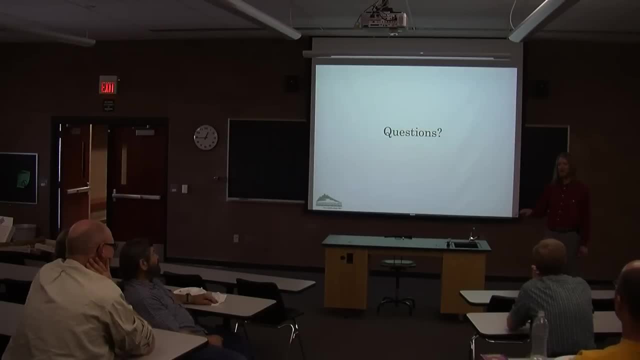 And again, from what I understand, that was not the direction that his employer wanted him to go in France, And so he came back to the United States in 1958, I think it was when he got his job with IBM, working in one of their research facilities. 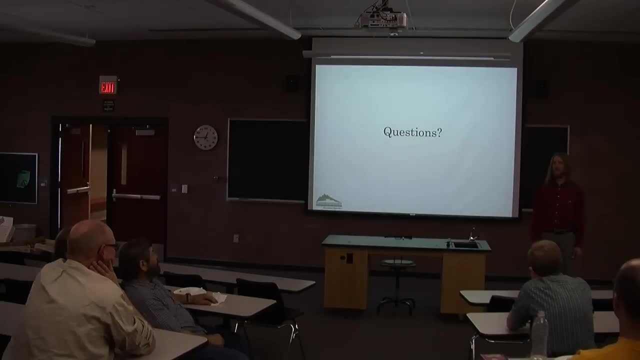 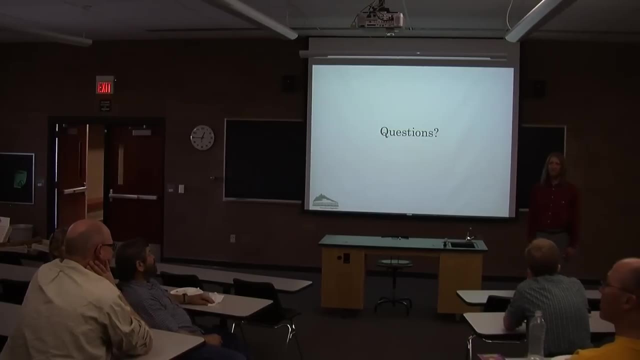 in New York doing specifically doing stuff with computers and modeling. Does that answer your question? Oh yeah, I've never read something about it, never read much more about it. Okay, that's it. So are there any other practical applications? 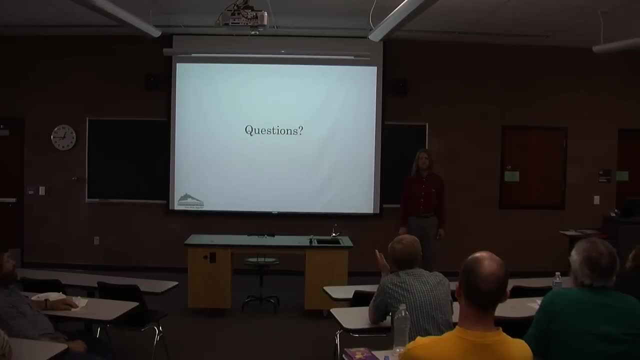 of the Dugner test besides, or his work besides, the Mandelbrot test. Well, my understanding is that these sets can be used to generate pseudo-random numbers. Does that sound right, Anybody, any of the computer folks? It can be used for, like cryptography applications. 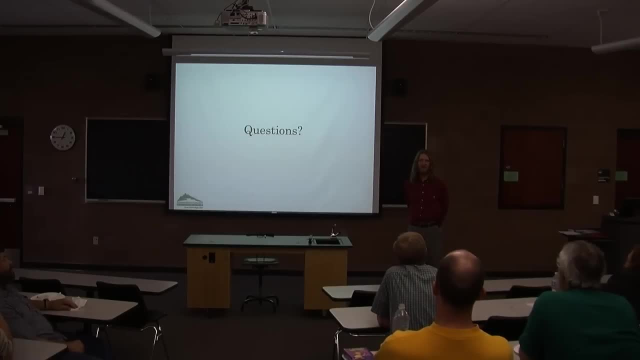 for generating sequences of random numbers, because there's no way to tell whether a particular point is going to be in the Mandelbrot set. So, even if- even I would guess- if your algorithm for picking points is not random, whether those points are in the Mandelbrot set or not, 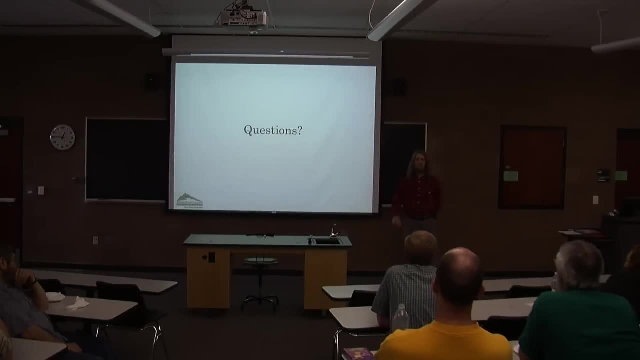 would be effectively a random sequence. Other than that, no, Yes, The unfolding of it seems to be almost like a mandala, Like a. what A mandala? Mandala, Mandala. I know, I guess I know what that is. 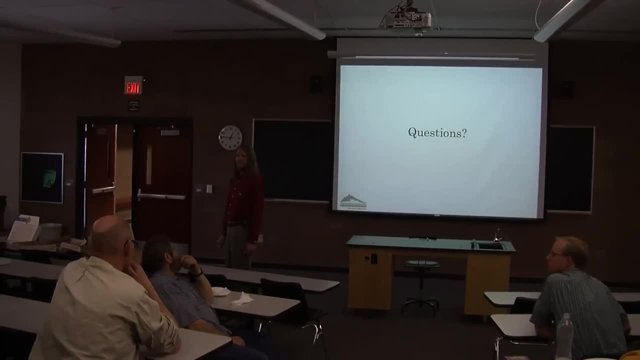 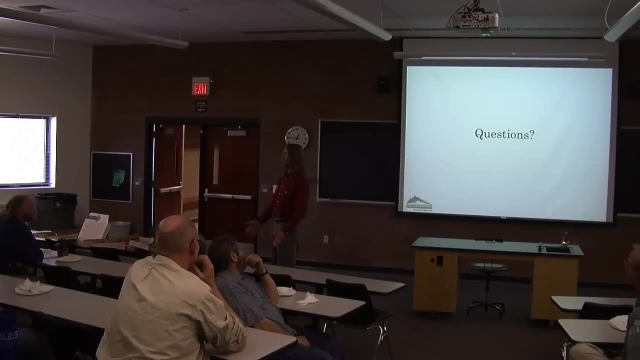 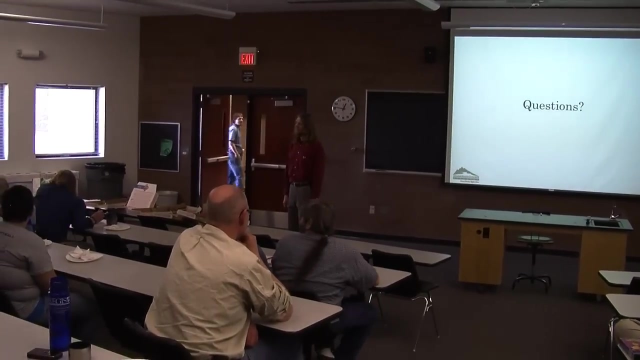 Just a hard question. I wanted to be able to suggest another thing. Those are mandalas, but not a mandala. Okay, I don't know anything about that to be able to say Well, but just the perpetual unfolding is part of the idea of the mandala. 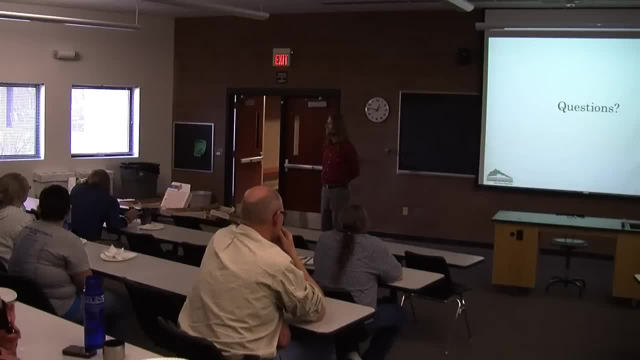 which is an ancient Christian religion, is this symbol which is kind of like a flower, a perpetual unfolding which generates perpetual energy. that occurred to me that the ancients might have been onto something in terms of some kind of esoteric understanding of this. 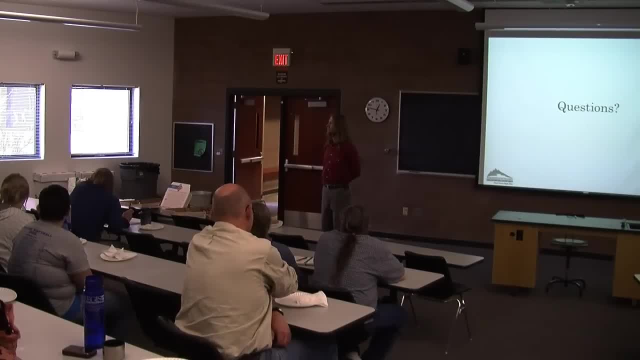 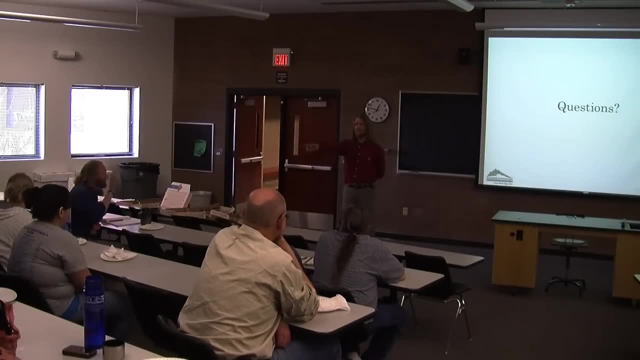 kind of like a quasi-foundation of ultimate reality. Is that possible? Yes, You said that the definition of chaos is the sense of. is it sensitivity to initial conditions or a way to describe chaos as a sensitivity to initial conditions? That's one of the recognizable hallmarks of a chaotic system. 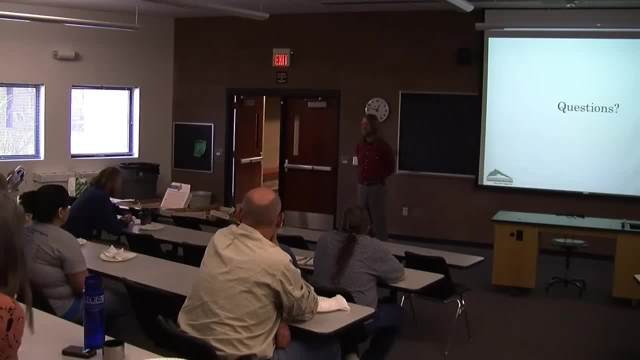 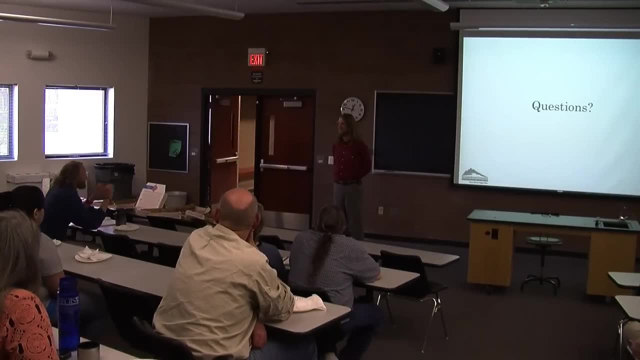 So in studying chemistry and kinetics we say that there's a rate law that describes how a reaction takes place and there's a sensitivity to the initial conditions And it depends upon the concentrations. to some power Right? Could that relate to chaos? 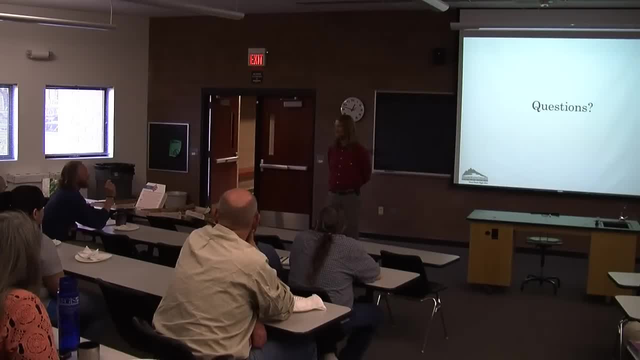 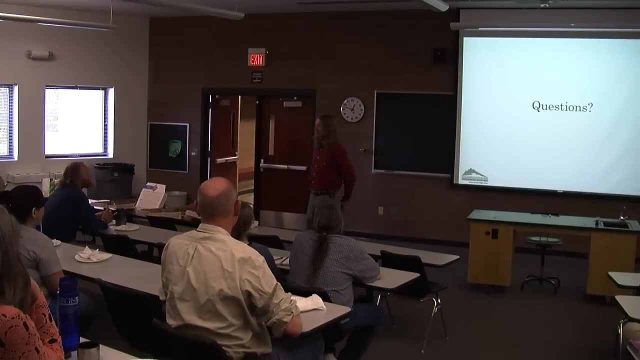 Do you know of anyone who has tried to examine chaos theory and rates of reactions and sensitivities and somehow relating numbers of microstates that are available? That's also an entropy. No, But most non-linear systems do exhibit some sort of chaotic behavior. 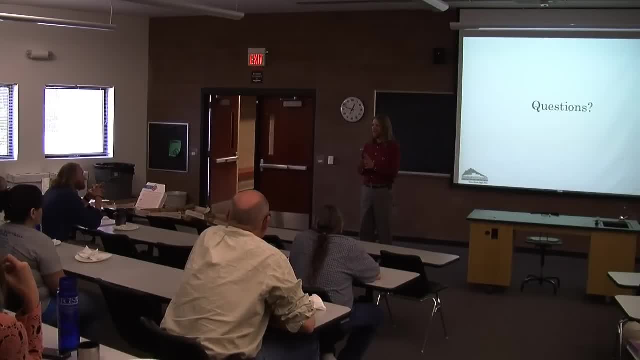 maybe not everywhere in their domain. They may not be sensitive to initial conditions everywhere. For instance, in an antelope set there's that big blob right around the origin that all of that stuff is in the Mandelbrot set. So within there a little bit of differences won't matter, right? 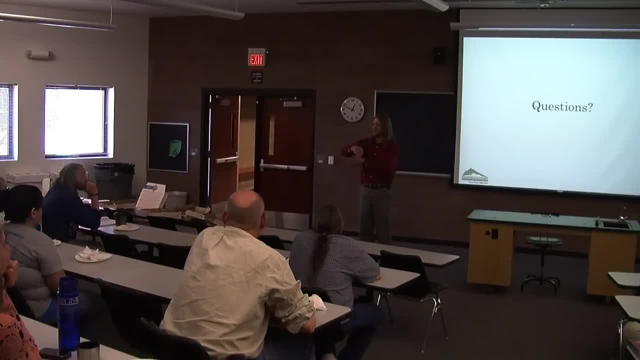 It's not that sensitive there. It's only on the boundary that it becomes very sensitive, And I think that depends on the system that you're looking at. But I do know that lots of people have tried to apply these ideas to various systems, but I don't know. 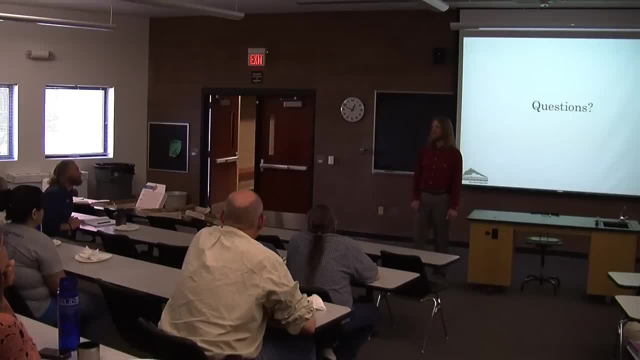 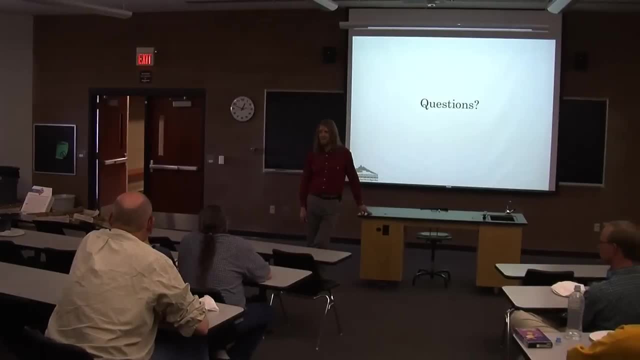 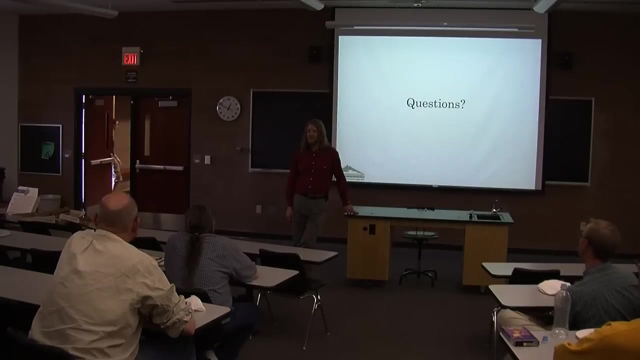 if anybody's really looked specifically at chemistry. My question's kind of related. I don't know what they're looking at. I think they're looking at the meteorologists that have the and they've taken into account this problem originally, or that Trevor was originally by a meteorologist.